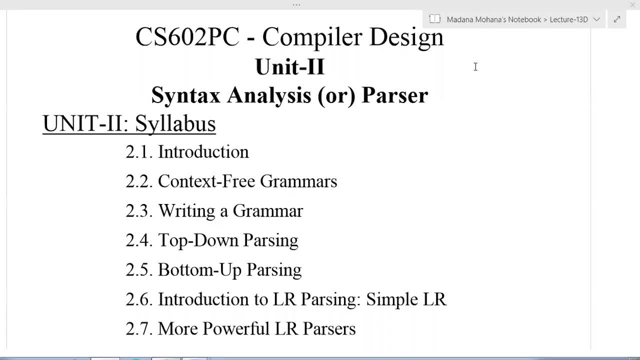 Welcome to the course Compiler Design. In this lecture we are going to start second unit, which is the second phase of compiler syntax analysis or parser. So in first unit we discussed about introduction to compilers, then pages of compilers, then compiler construction tools, Then later we studied the first phase which is called as lexical analysis. also, 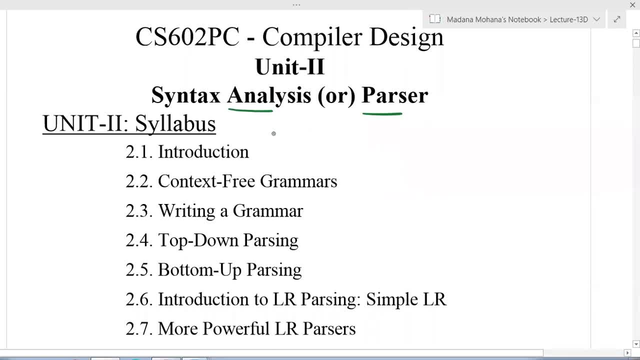 called as scanner. So now we will continue with the second phase, which is called as syntax analysis or parser. So in syntax analysis or parser we are going to cover the following topic: First we will see the introduction about syntax analysis or parser, then context-free. 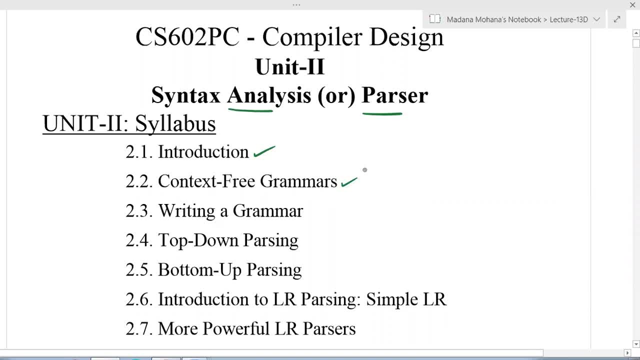 grammars same as formal language and automata theory. So in parser or syntax analysis context-free grammar Grammars are used, like in lexical analysis or scanner. finite automaton and regular expressions are used. So here context-free grammars are used. Then writing a grammar here eliminating 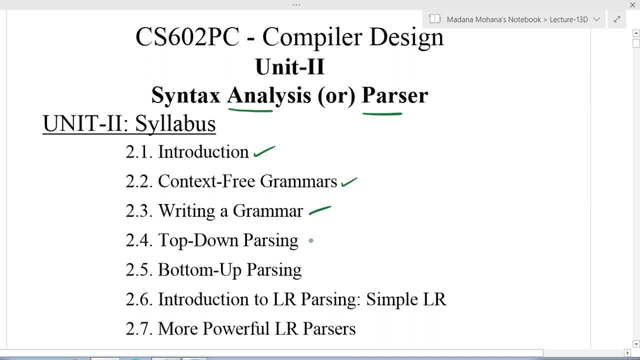 ambiguity and removing some other factors. Then syntax analysis or parser, consisting of two types: One is top-down parser, another one is bottom-up parser. So we will study these two. Then, in bottom-up parser, one of the technique which is called as expression: 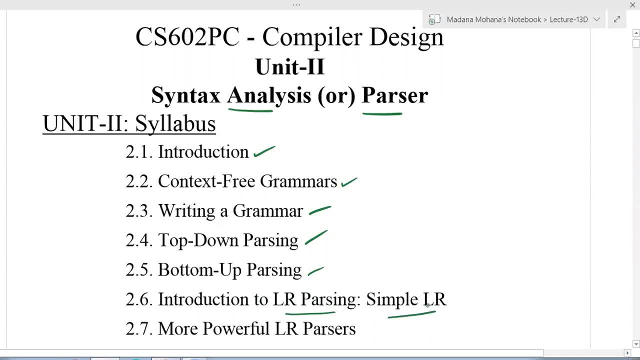 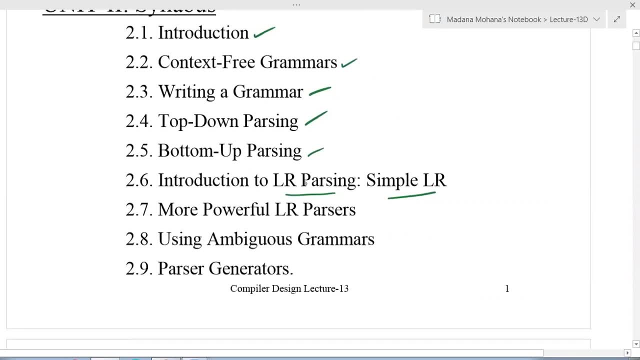 parsing. So here we will discuss about various types of LR parsers, like simple LR, then canonical LR, look-ahead LR- So many parsers are there- Then comparison of LR parsers, then using ambiguous grammars, then finally parser generator. Here parser generator is nothing but YACC. 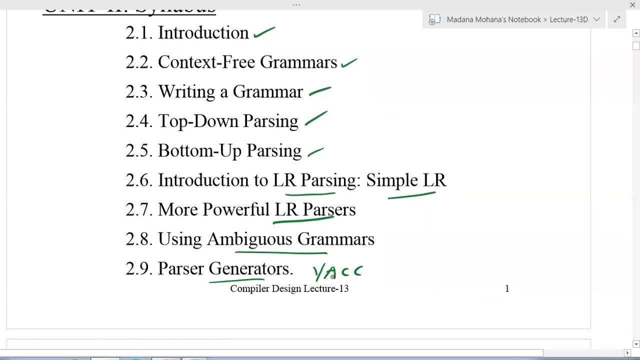 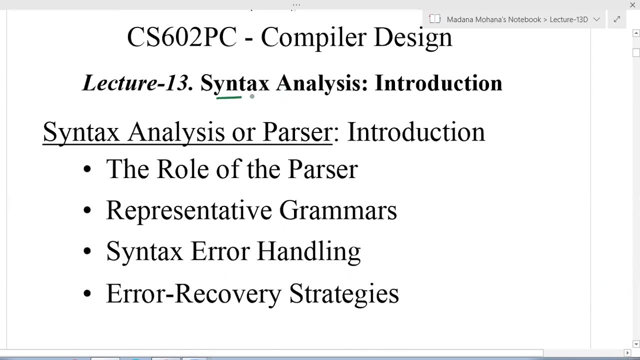 yet another compiler compiler. Like lexical analyzer generator, we have lex tool. Like parser also we have Generator, so which is called as YACC, yet another compiler compiler. So now in this lecture first we will discuss about introduction to syntax analysis. So in introduction first. 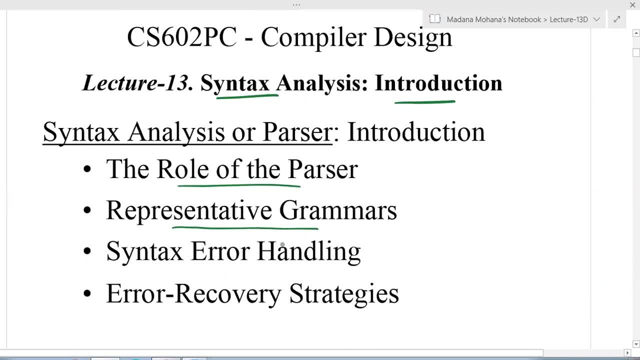 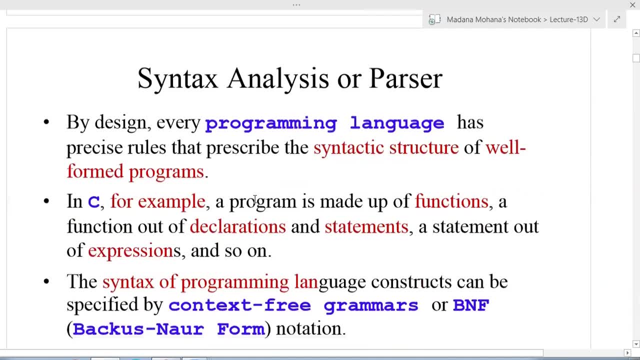 we will see the role of the parser, then representative grammars, then syntax error handling, then various error recovery strategies. So now you can recall once the phases of compiler in that we discussed a little bit. So now you can recall once the phases of compiler in that we discussed a little bit. 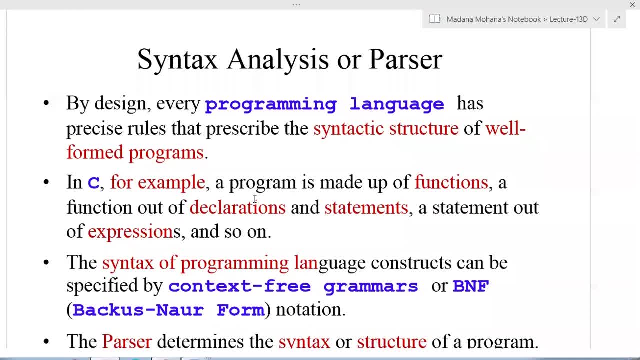 about the introduction, about the phases of compilers as well as each phase. So syntax analysis and parser. also we discussed syntax analysis, parser, which takes input as the output of lexical analysis, that is token. then syntax analysis or parser can represent the tokens into hierarchical form which is called as a tree, that is called a syntax. tree, or derivation tree, or parse tree, and here we can see a hand, Zhuang61護, and we can see a very interesting저 and we can see how, basically, lash tree is pointed to stdef, complex Right. so now this Lemme introduce you now this little bit of the phases of compilers as 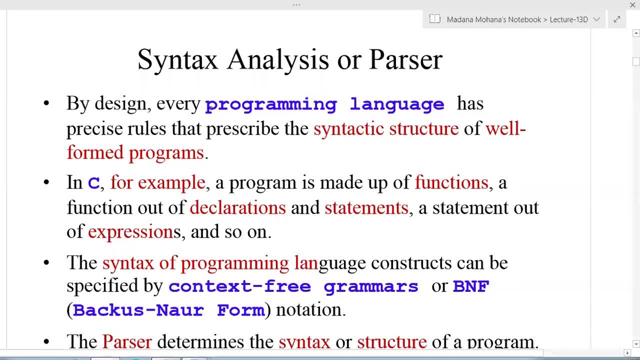 So that is the output of syntax analysis at parser. So by design, every programming language has precise rules that prescribe the syntactic structure of well formed programs. For this purpose, for example, in C language a program is made up of functions. a function- 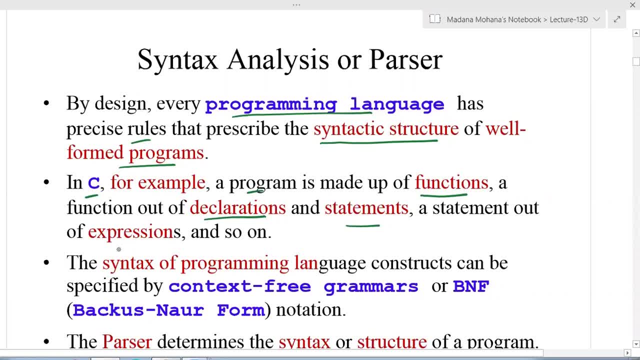 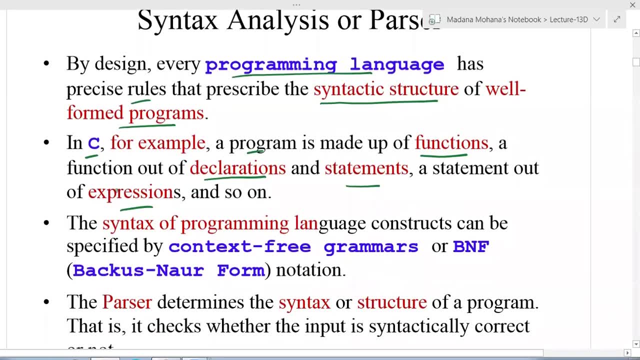 out of declarations and statements, a statement out of expressions and so on, like all these combinations. Now, the syntax of programming language constructs can be specified by using context-free grammars. So also BNF notation, that is Bacchus-Nor-Form notation, So actually, 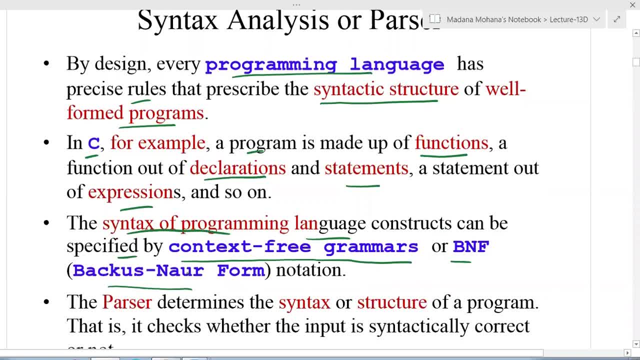 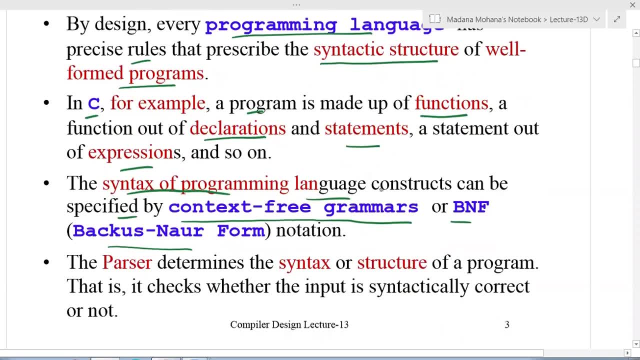 the grammar syntaxes can be defined by using BNF notation. Now, this is the use of context-free grammars. here The syntax of programming language constructs can be specified by context-free grammars or BNF notation. The parser then determines the syntax structure of a program, that is, it checks whether the input is syntactically. 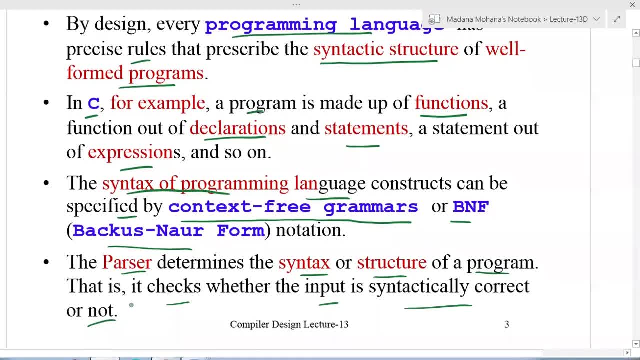 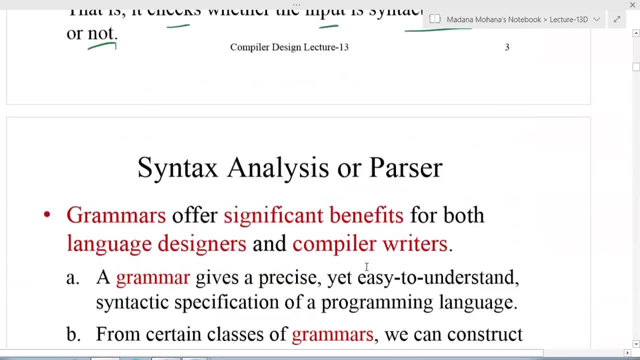 correct or not. So this is the role of the parser: it checks whether the input is syntactic correctly or not. So the syntax structure of a program. So then, grammars offer some significant benefits. SUE LAWORTIME, SPACEVALUES, Sharcroости. Nadeem AurBookavic discipline course http//t. siparistncelelde. 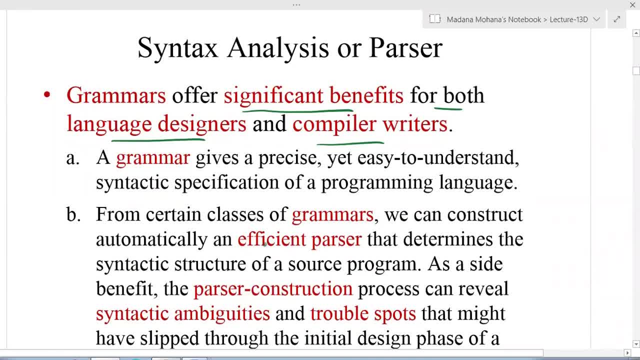 language designers and compiler writers. Now, what are those benefits? A grammar gives a precise, at easy to understand, syntactic specification of a programming language. This is one of the advantages. So grammar advantages for both language designers and compiler writers. The second advantage: from certain classes of 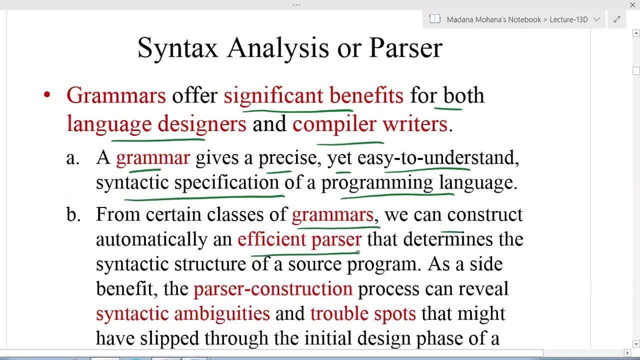 grammars we can construct automatically an efficient parser that determines the syntactic structure of a source program. So with the different classes of grammars we can construct automatically with an efficient parser further that determines the syntactic structure of a source program. As a side benefit, the 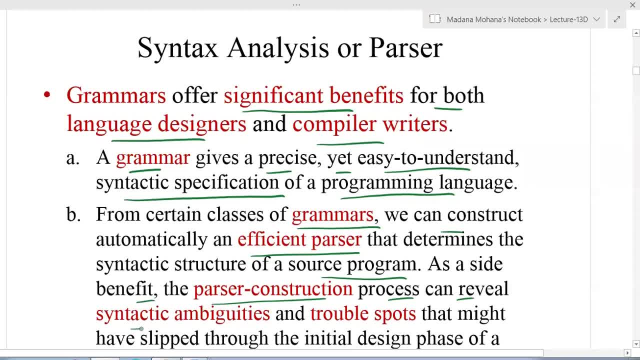 parser construction process can reveal syntactic ambiguities and trouble problems. We can also identify errors in the structure of a grammar, So a grammar is an important part of a structure that can be used to identify errors. A grammar is a structure that can be used to identify errors. 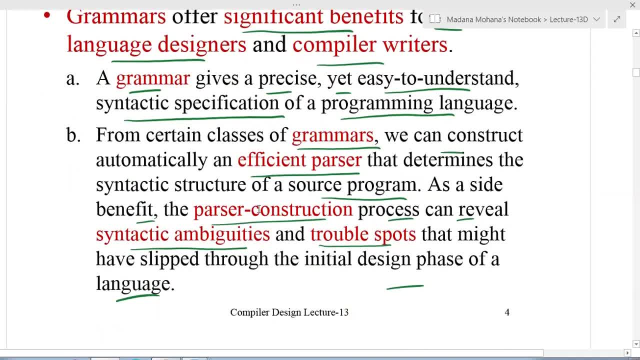 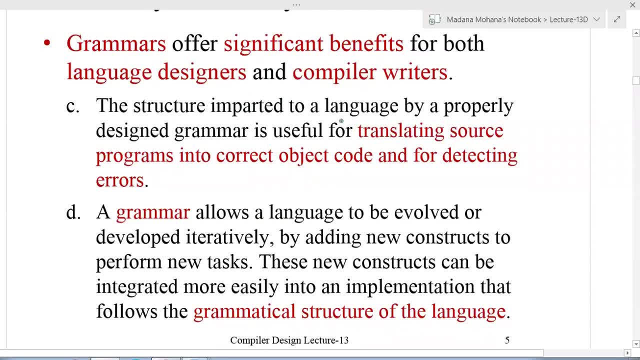 So here identification of errors, So for that also grammars plays an important role. So next one: the structure imported to a language by a properly designed grammar is useful for translating source program into correct object code and for detecting errors, Like the role of compiler transforming the source program into other form, But the other form is in correct object code, and for detecting errors. 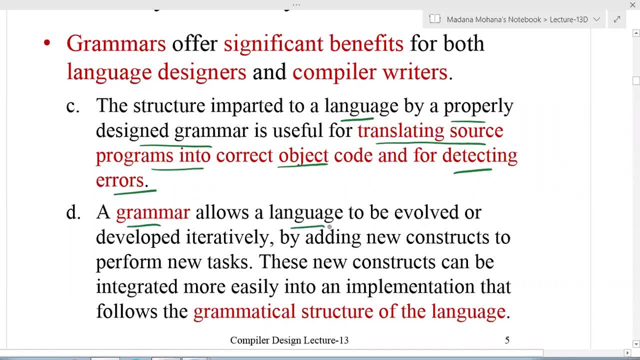 Then another advantage: a grammar allows a language to be evolved or developed iteratively, repeatedly, by adding new constructs to perform new tasks. These new constructs can be integrated more easily into an implementation that follows the grammatical process. This is the grammatical structure of the language. 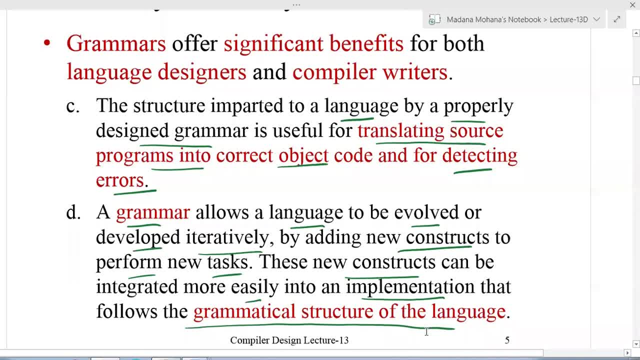 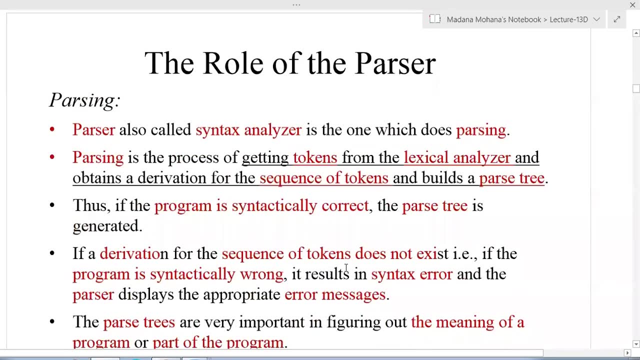 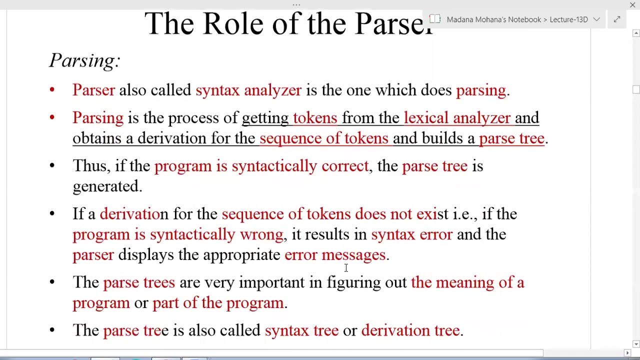 So from one grammar to designing some new constructs by integrating, So those are all useful for implementation of the grammatical structure of the languages. So these are all the advantages of grammar for both compiler writers and designers. Now coming to the role of the parser. 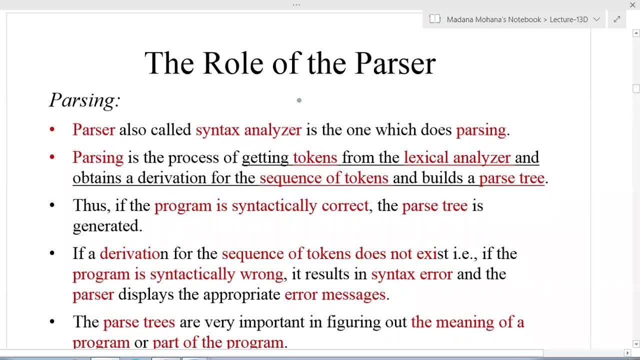 So the role or position of the parser in the pages of compiler. So now onwards, in place of syntax analysis, parser will call it, as I mean. syntax analysis will be called as parser. Now the approach is called as parsing. How to define a parser? 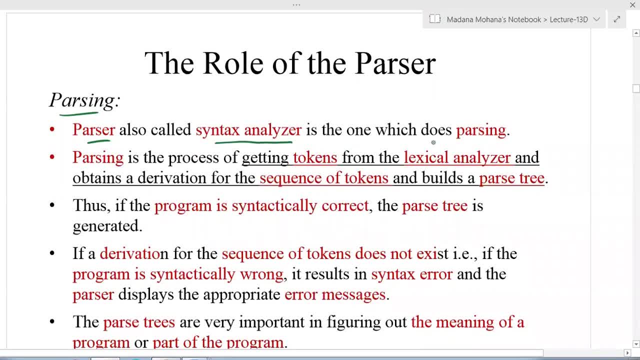 Parser, also called syntax analyzer, is the one which does parsing. Parser or syntax analyzer will do parsing. Parsing means derives. It derives the strings based on that derivation. who can take decisions? The string is derived or not? Now, what is the definition of parsing? 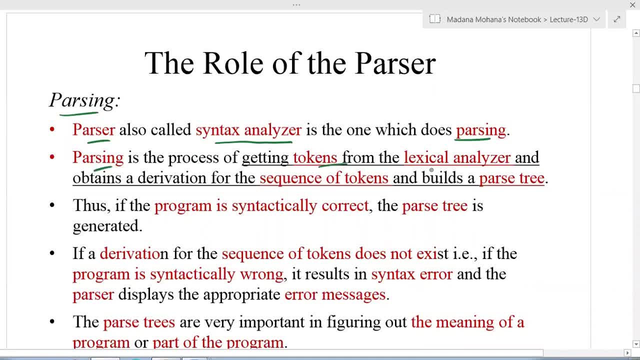 Parsing is the process of getting tokens from lexical analyzer and obtains a derivation for the sequence of tokens and builds a parse tree. This is the concept of parsing, So it is the process of getting tokens from the lexical analyzer which is output of lexical analyzer or scanner. 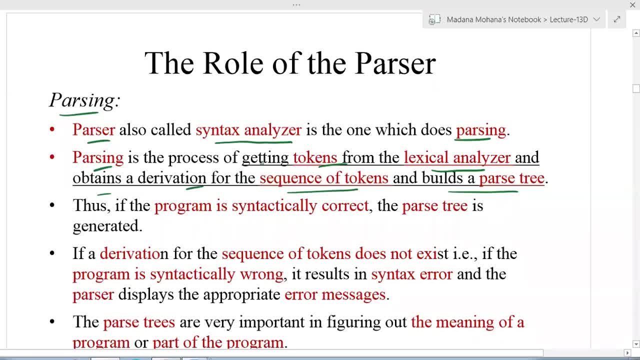 And obtain a derivation for the sequence of tokens From the tokens. it derives sequence of derivations from the sequence of tokens and further builds a parse tree That is the hierarchical representation Parse tree, also called as derivation tree. Thus, if the program is syntactically correct, the parse tree is generated. 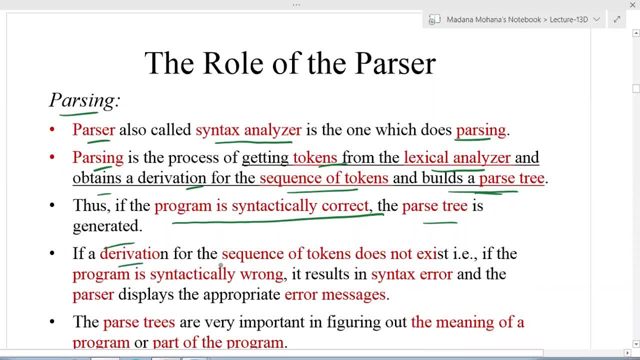 Otherwise the parse tree won't generate it. If a derivation for the sequence of tokens does not exist, that is, if the program is syntactically wrong, it results in syntax error and the parser displays the appropriate error messages, Like in a first-phase lexical analysis or scanner. also it encounters errors. that is lexical error. 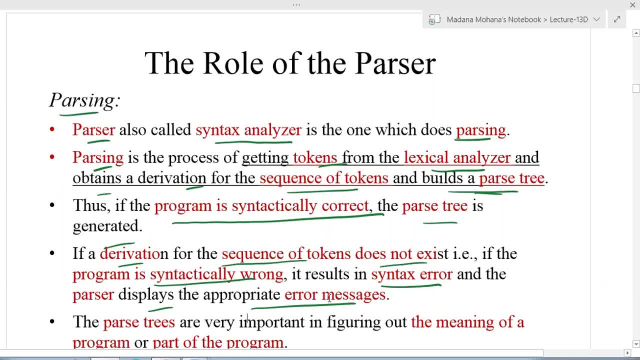 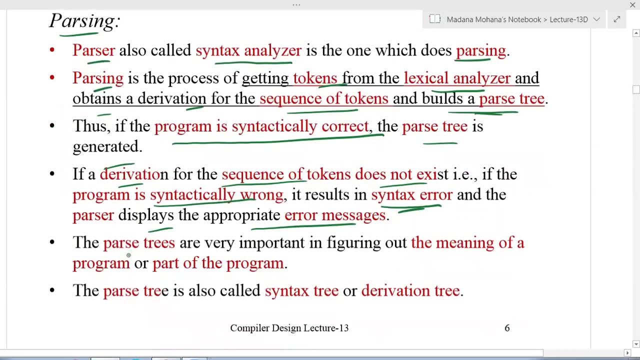 Then how to handle lexical error. So we discussed in lexical analysis, Whereas in parser or syntax analysis also, errors are encountered, These errors are called as syntax errors. Then how to handle these syntax errors That we will cover in this lecture. So now finally, the parse trees are very important in figuring out the meaning of the program or part of the program. 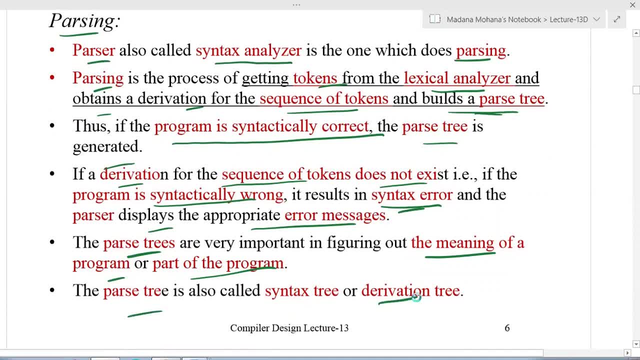 That is, use the parse tree. Now parse tree is also called as derivation tree generally, Then syntax tree. But syntax tree, parse tree, there is slight difference we discussed in earlier lectures. Syntax tree does not require grammar, Only string is required. 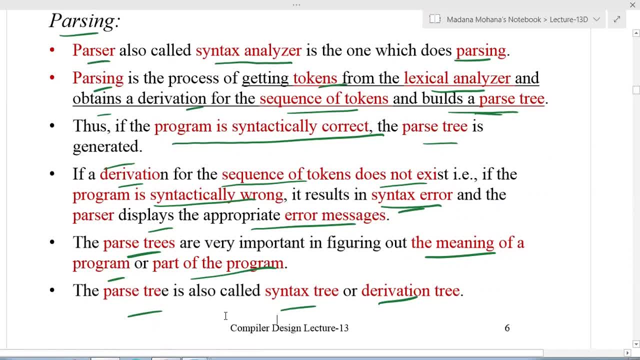 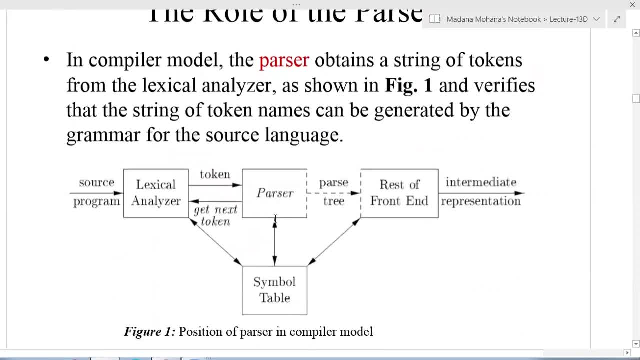 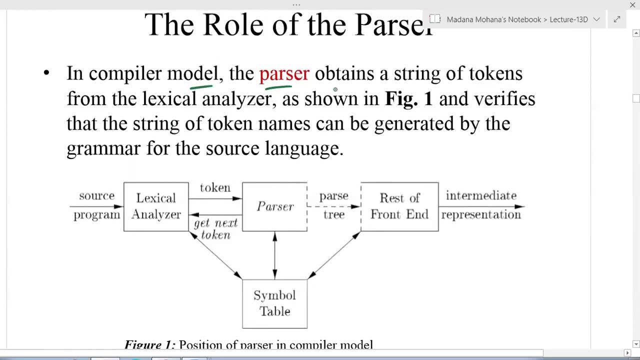 But parse tree or derivation tree, grammar is required. That is the major difference between parse tree and syntax tree. Now let us see the role of the parser. So that can be shown in the following diagram. In compiler model, the parser obtains a string of tokens from the lexical analyzer. 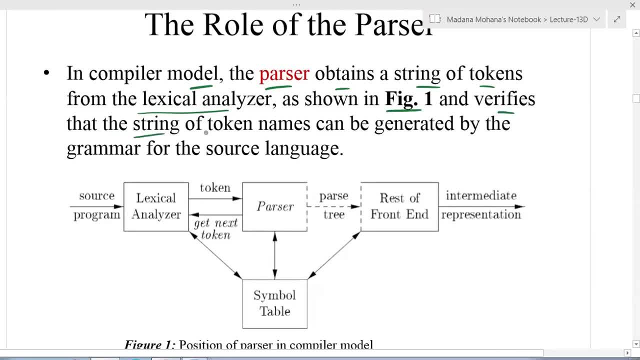 As shown in figure 1.. And verifies that the string of token names can be generated by the grammar for the source language. So this is the role of the parser. Now diagrammatically you can see. So for lexical analysis also, we discussed the role of the 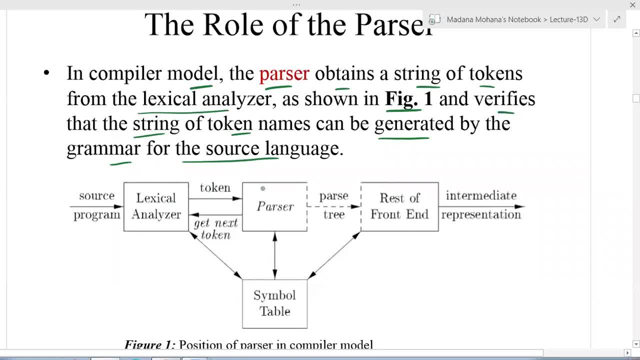 Lexical analysis or scanner. So that part of the diagram is here itself. It is included Now. this is a lexical analyzer which takes input as the source program then produces token. That token is taken as input to the parser. Then whenever parser wants next token, using the method get next token, it takes the next parser. 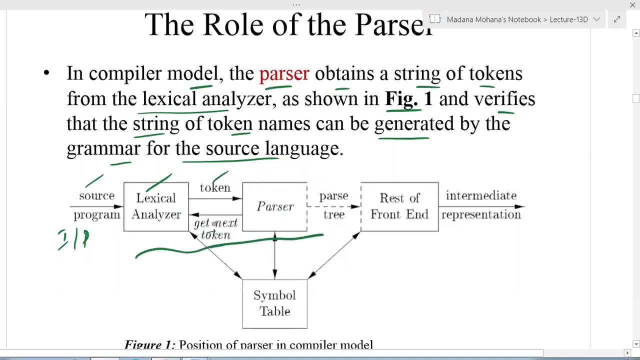 So up to this, up to this, that is the role of the lexical analyzer. Now we are discussing about Parser. the role of the parser with the same previous lexical analyzer part is continued now from parser. Here you can see the output of parser is parse tree with the hierarchical representation. 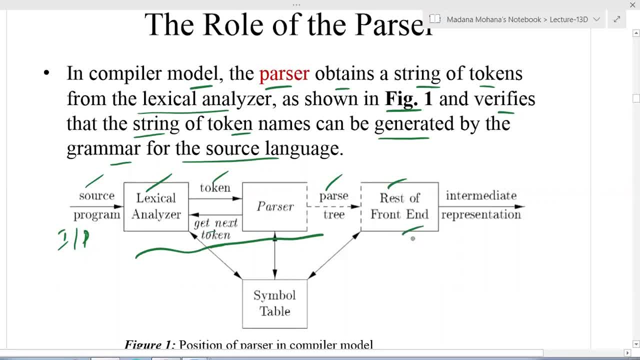 So latter rest of the content, other pages like semantic analysis, then intermediate code, code optimization, code generation. Those are all the backend pages. Finally, here you will get a semantic analysis. Is that The third phase of compiler semantic analysis which produces abstract syntax tree? then that will be taken input to the next two phase. 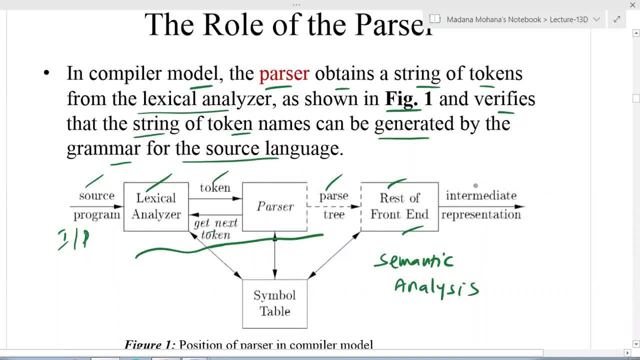 That is, intermediate code generator. So in the form of intermediate representation now you can see symbol table is connected to all the phases. So in the phases of compiler or block block diagram we can recall all phases are connected to symbol table and error handler. 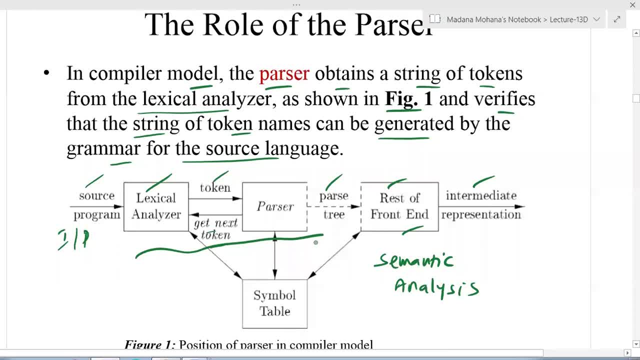 Each phase encounters error, So those errors are handled by using the respective phase error recovery strategies. So these are diagrammatic representation of the role of the parser Here. parser takes token from the lexical analyzer, then produces derivations. from the derivations It constructs a parser derivation tree. 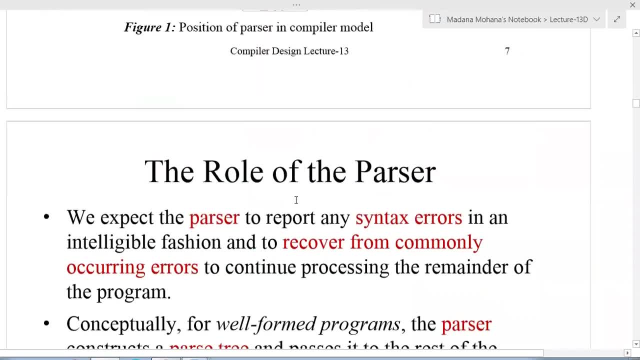 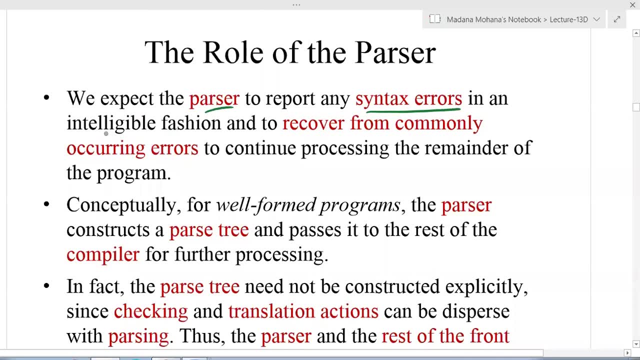 That is the role of the parser. So now here We expect the parser to report any Syntax errors in an intelligible fashion and to recover from commonly occurring errors, to continue processing the remainder of the program. So, conceptually, for well formed programs, the parser constructs a parse tree and passes it to the rest of the compiler for further processing. 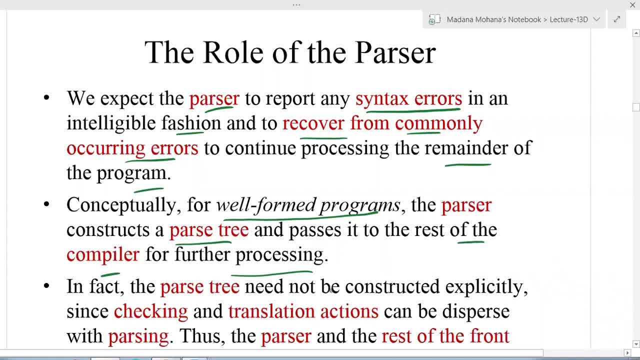 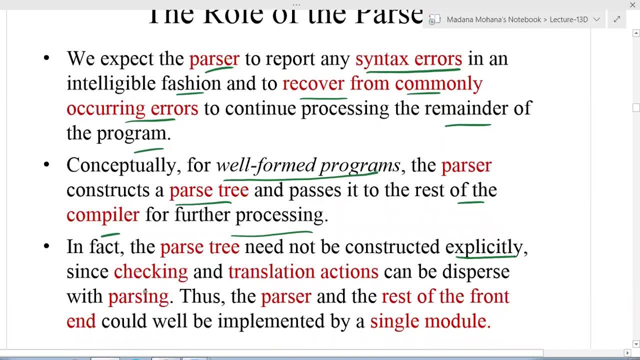 That is the front end, the rest of the part followed by backend. In fact, the parse tree need Not be constructed explicitly, Since checking and translation actions can be dispersed with parsing only Does the parser and rest of the front end would well be implemented by a single module. 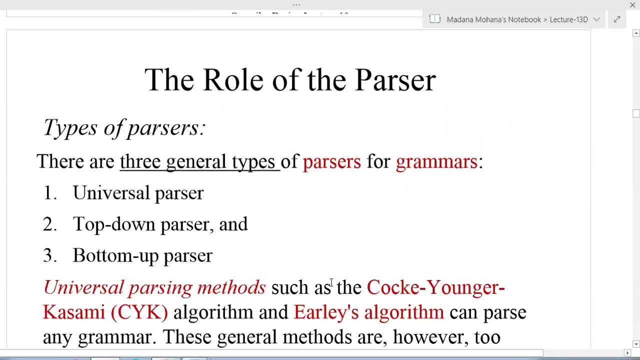 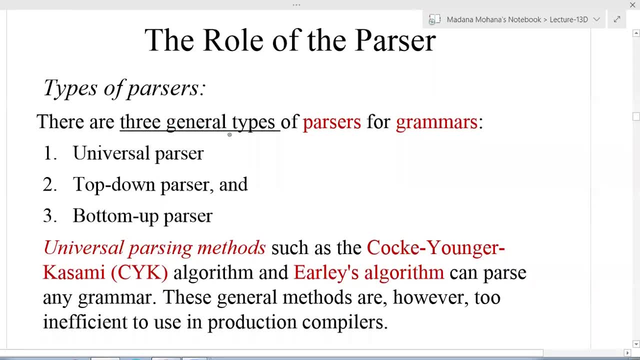 That is the advantage of the parser. So now there are various types of parsers or parsing techniques. So there are generally three general types of parsers for grammars. The first one is It's called a universal parser. Second one is called a top down parser. 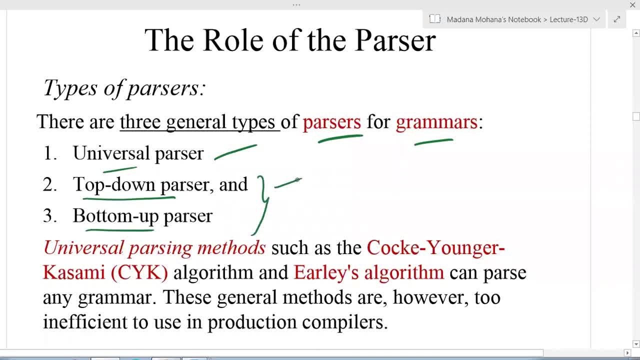 Third one is called a bottom up parser. As for syllabus, we'll discuss about in detail, with all the techniques of these two types of parsers, That is, top down parser and bottom up parser. The universal parser is nothing but Some of the universal parsing methods, such as CYK algorithm in formal language and automata theory membership algorithm we discussed in context with languages. 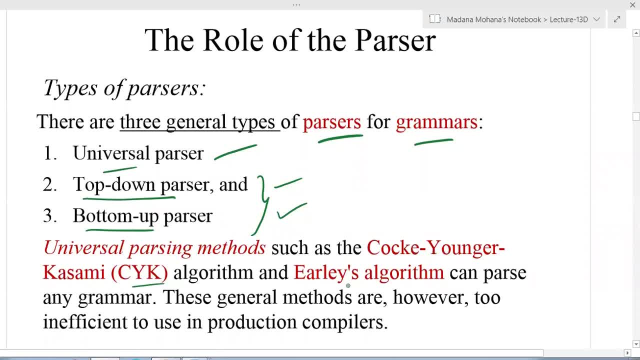 So that is CYK, Coq, Angle, Casami And other algorithm Early algorithm, So both these algorithms can parse any grammar. These general methods are, however, too inefficient to use in production compilers, So this is the universal parser. 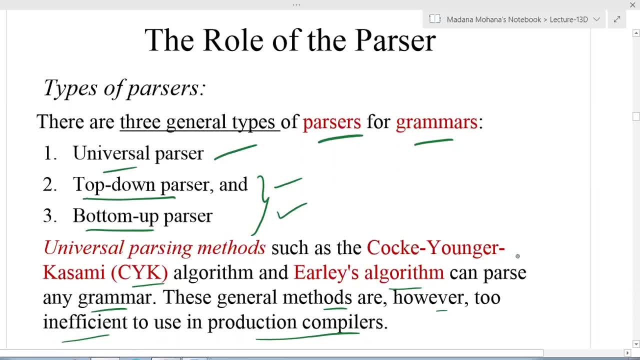 So here this we want to study here CYK anyway. we already discussed in formal language and automata theory. So other algorithm, early algorithm. both algorithms can parse any grammar, But these general methods are too inefficient to use in production compilers. 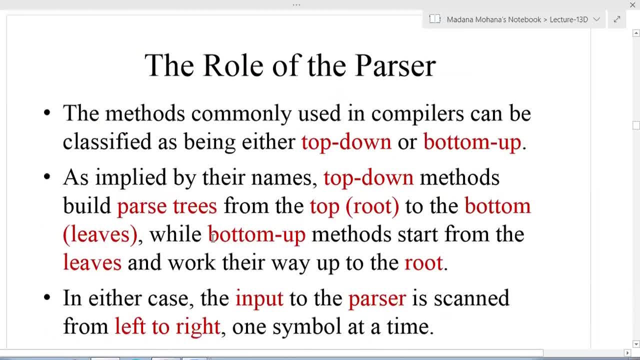 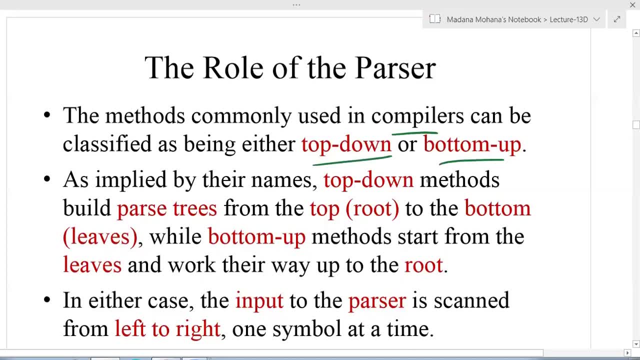 So now let us come to top down parser and bottom up parser. These two are very important. The methods commonly used in compilers can be classified as being either top down parser or bottom up parser. Now, what is top down parser as implied by their name? top down method: build parse tree from top root to bottom leaves. 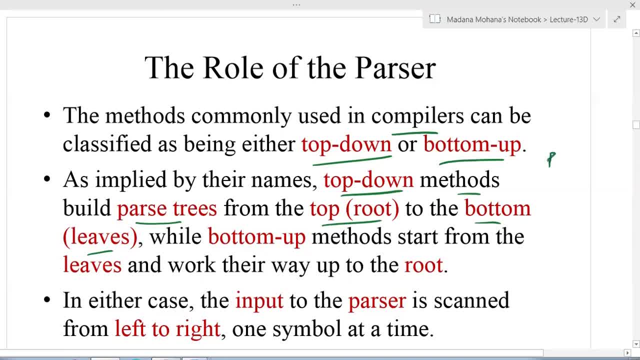 So construction of A parsed tree or derivation tree, from starting from root, then proceed towards leaves, that is the leaf node. This is called as top down parser, whereas bottom up parser. so starting with the leaf nodes, then you can derive its root. 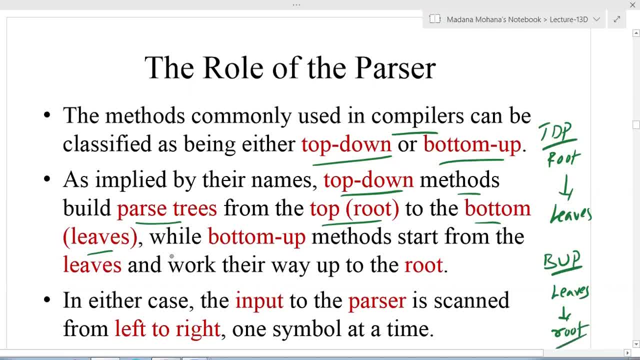 This is called as bottom up parsing. So now the bottom up while bottom up method starts from the leaves And work their way to the root. So simply you can identify: top down parsing is nothing but root to leaves, whereas bottom up parsing is nothing but leaves to root. 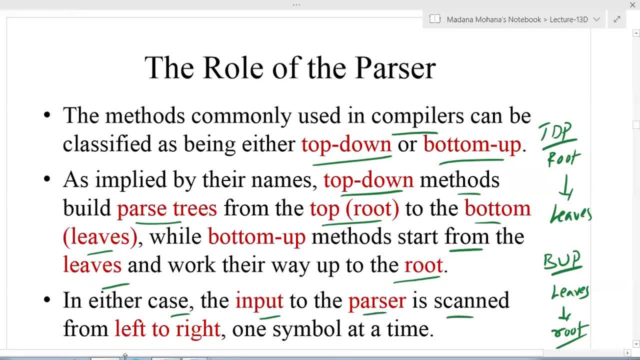 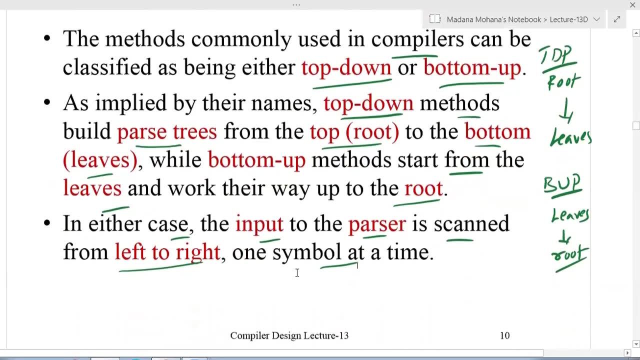 In either case, the input to the parser is scanned from left to right, only only one symbol at a time. So this is the condition of reading of the input: So from left to right, one symbol at a time. So these are all the two types of parsers: top down parser and bottom up parser. 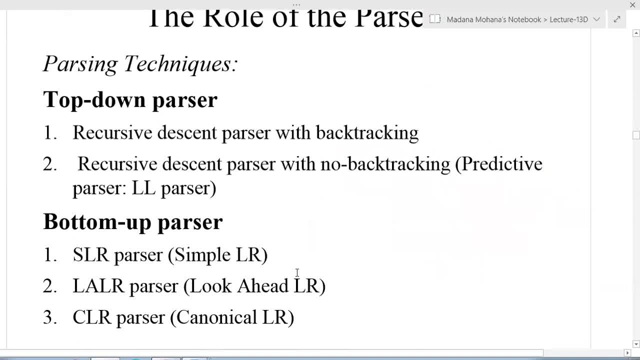 So now, before proceeding further here itself, now we will list the parsing techniques. So these are all very important. In syntax analysis syllabus we'll study about all these techniques related to the two types of parser. First, for top down parser, we are having two techniques. 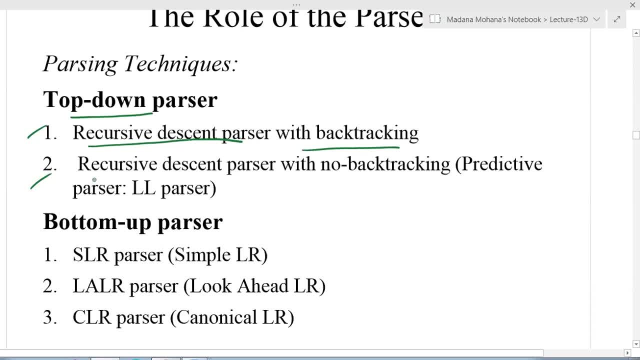 First one is recursive descent parser with backtracking, Then recursive descent parser with no backtracking, So this technique is called as Predictive parser, which is called as LL parser. So in top down parser, we'll discuss these two techniques Here. predictive parser- LL1. 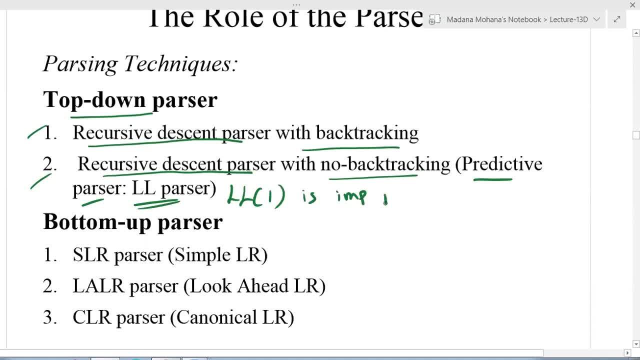 So is important problem. So in examination we will expect this question: LL1 parser Then, whereas bottom up parser. So three techniques are there. First one is SLR parser means simple LR, Then LLR parser means look ahead, LR parser. 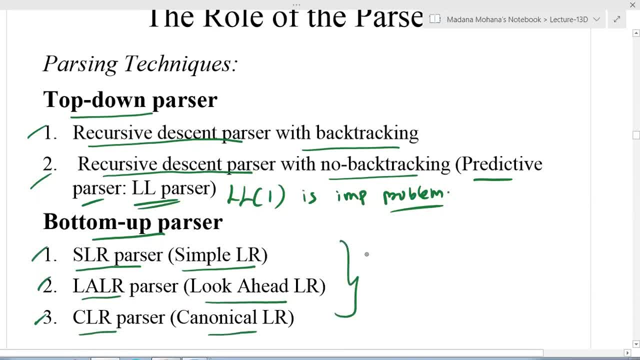 Then CLR parser means canonical LR parser. So here for every parser we'll discuss about- Here you can see SLR1 parser, LALR1 parser, Then CLR1 parser. For all these we'll discuss about algorithm, Algorithm. 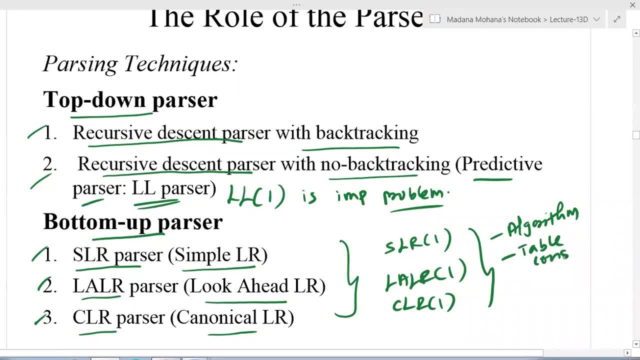 Then parsing table construction. Parsing table construction, Then parsing How to do parsing. So these three For every technique. we'll discuss about these three topics: Algorithm table construction, then parsing For LL1, also LL1, also Algorithm table construction method, then parsing with example. 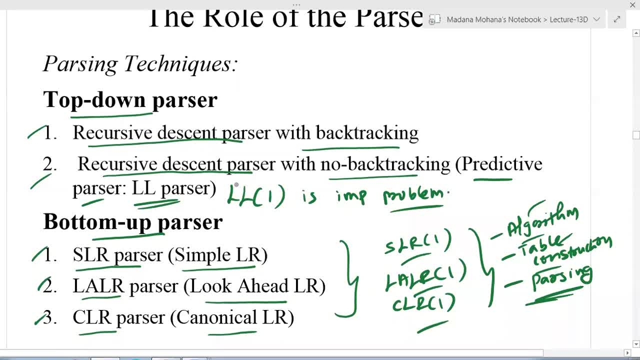 So entire of the second unit, The three plus one, four topics, So related to problems. So definitely you will get One or two questions. If it is a choice based, we'll get two questions. But you have to concentrate more on this year for all these topics. 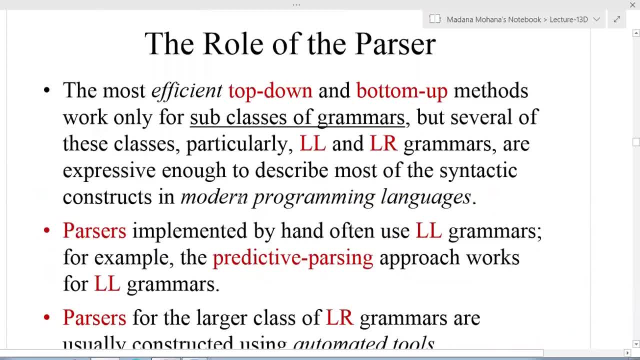 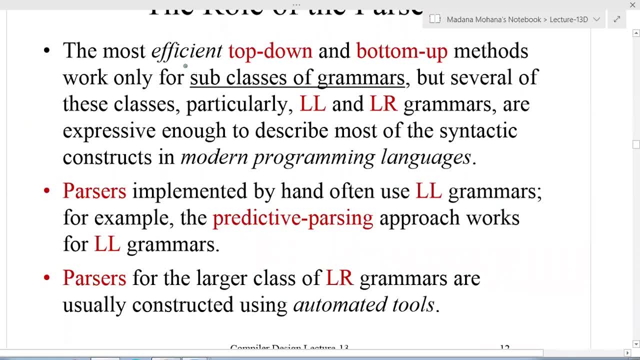 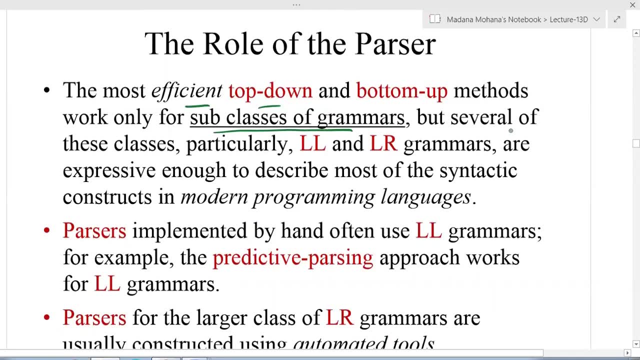 Continuity is required Now. So let us compare these two with some Efficient measures. The most efficient top down and bottom up methods Work only for subclasses of grammars, But several of these classes, particularly LL, That is, the predictive parser, part of top down parser, and LR grammars- 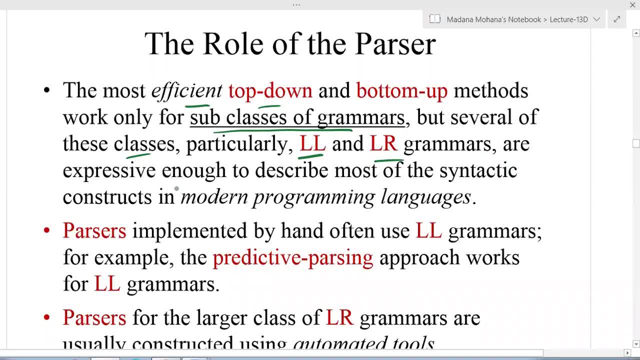 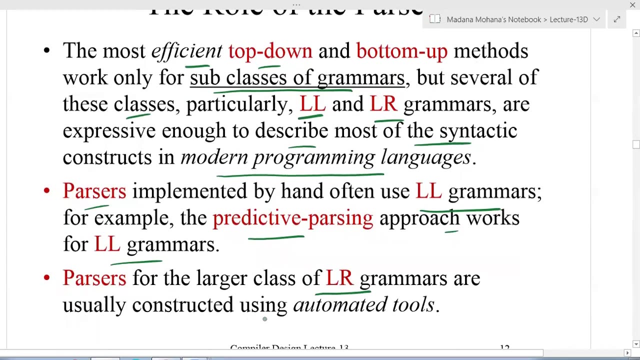 That is bottom up parser. So these two are expressive enough to describe most of the syntactic constructs in modern programming languages. Parsers implemented by hand often use LL grammars, For example. the predictive parsing approach works for LL grammars, Whereas parsers for the large class of LR grammars are usually constructed. 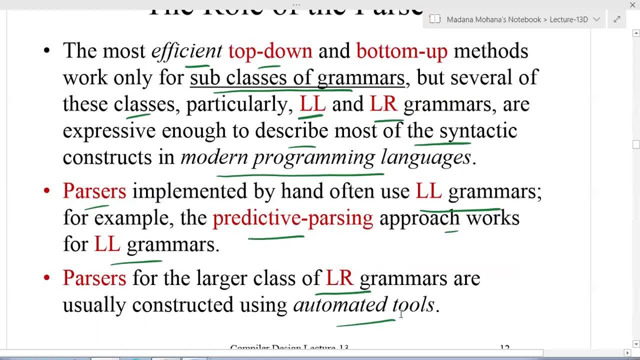 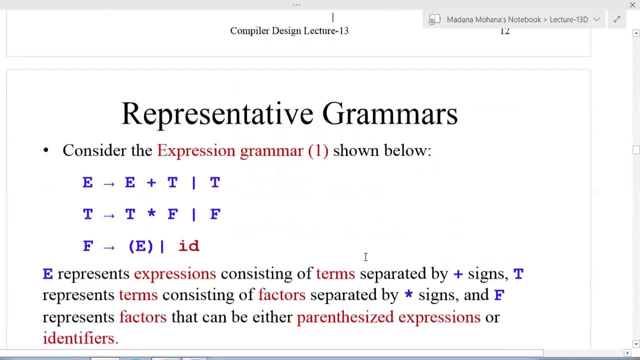 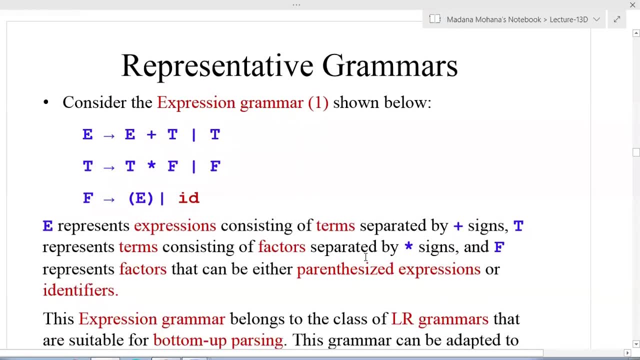 Using some automated tools, like we have YSAC, parser, automatic generator tool at another compiler, compiler. So then coming to representative grammars. So here for parser, for construction of derivation tree or parse tree, Then for describing programming language constructs, compulsory grammar is required here. 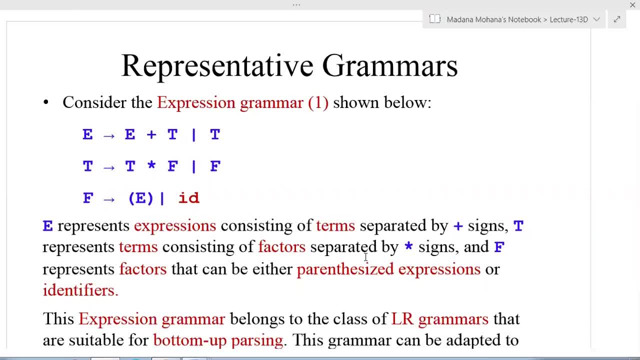 So here, what type of grammars are used. Now consider the expression grammar: arithmetic expression grammar, To name it as one shown below. So earlier also we discussed this example During the formal language and automated theory discussion of context tree grammar. So arithmetic grammar or expression grammar is defined as: 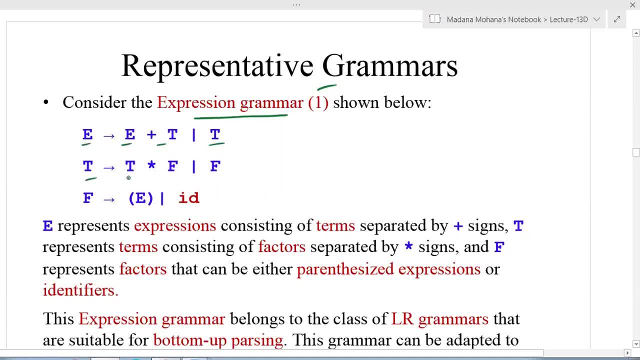 So E derives E plus T or T, Then T derives T into F or F, Then F derives E within parentheses or ID. Here C plus is the arithmetic operator, Then star is the multiplication operator. So now here: E stands for expression. E stands for expression. 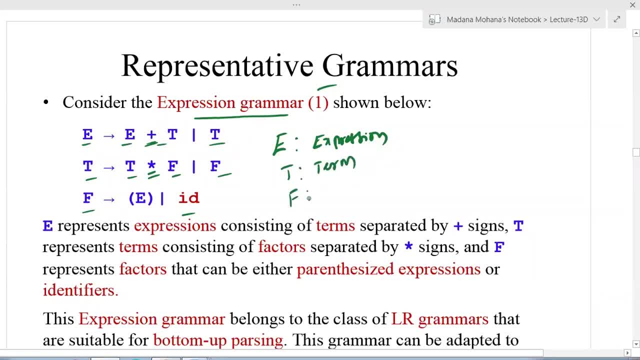 Then T stands for term, Then F stands for factor, So now that E represented within parentheses, Then, whereas ID, which can be denoted with boldface, character Which is called as identifier, So in grammar we know- G equal to V, T, S, P. 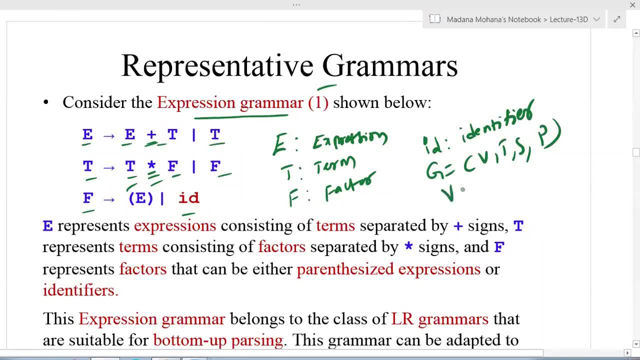 Defined with portables, Where capital V is nothing but set of variables. Here the variables are E, T, F, So that is expression, term and factor. Then, where our terminals are The operators, plus into Then the parentheses: open parentheses, closed parentheses. 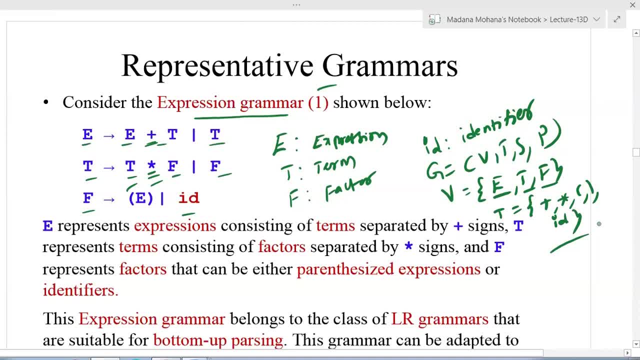 Then ID. These are all the terminals of this grammar. Then, whereas Starting variable S is E, Why? Because the first production left hand side symbol is called a starting variable. Then productions are: These are all the productions given. So this is one example of expression grammar. 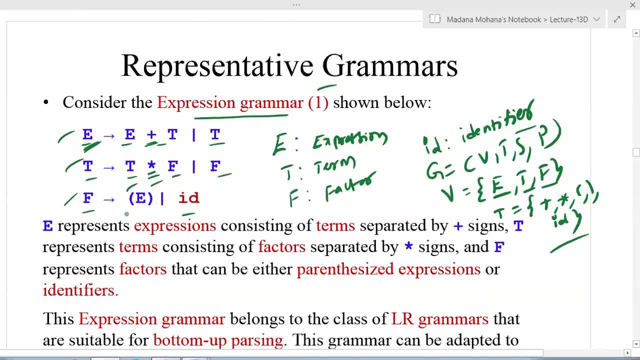 So we will use In syntax analysis or parse. Here E represents expression consisting of terms separated with plus sign, Then T represents terms consisting of factors separated with star. Then F represents factors That can be either parenthesized expression within parentheses Or identifies what we discussed here. 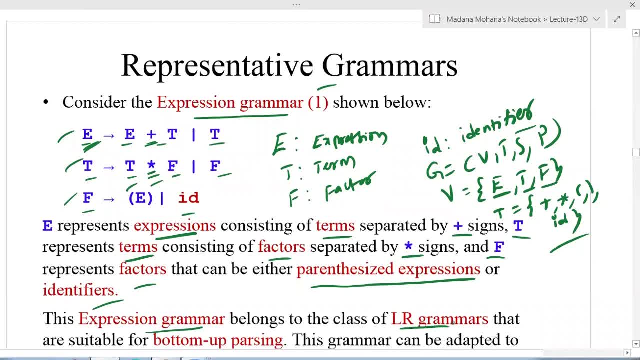 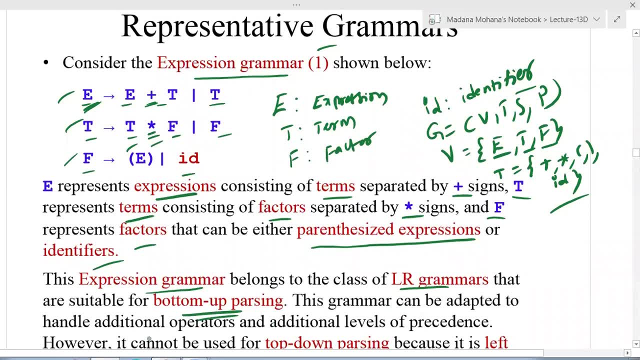 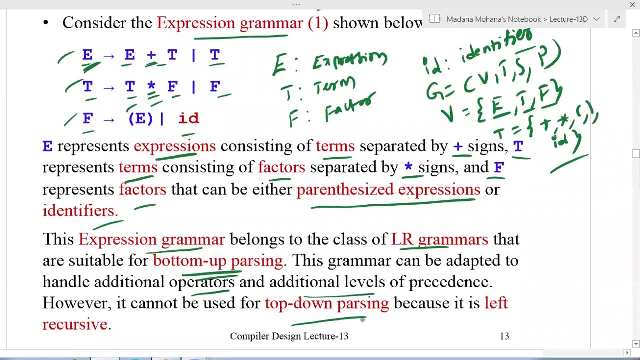 This expression grammar belongs to the class of LR grammars Which are suitable for bottom up parsing, So this grammar can be adopted to handle additional operations And additional levels of precedence. However, It cannot be used for top down parsing Because it has left clickers U. 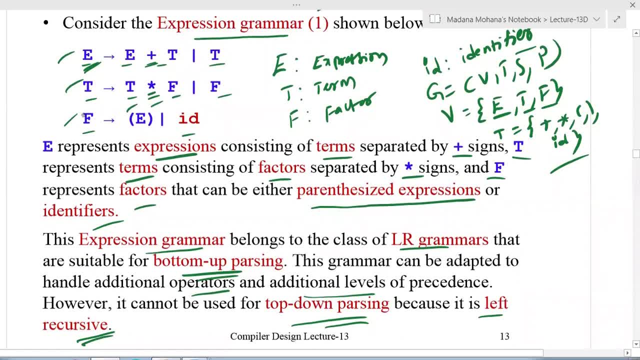 So here this example grammar Is suitable for bottom up parsing Or not suitable for top down parsing Because it has left recursion. So the left recursion concept is nothing but Left hand side Symbol is same as in the right hand side, Left most symbol. 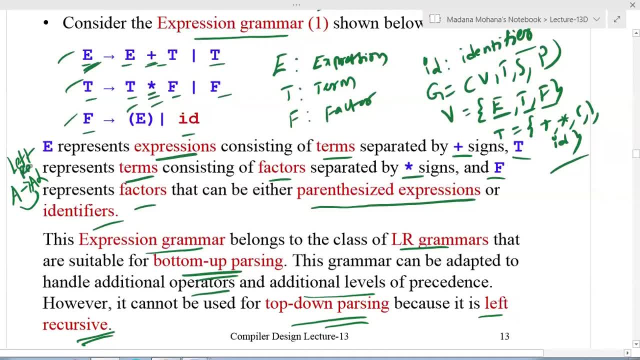 If these two are same Then this is called as Left recursion. Now in top down parser, if any grammar having left recursion we have to eliminate, That we will discuss later In the upcoming concepts. So The grammar without left recursion That can be used for top down parsing. 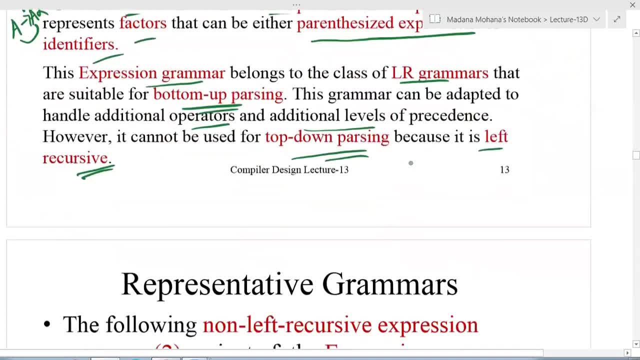 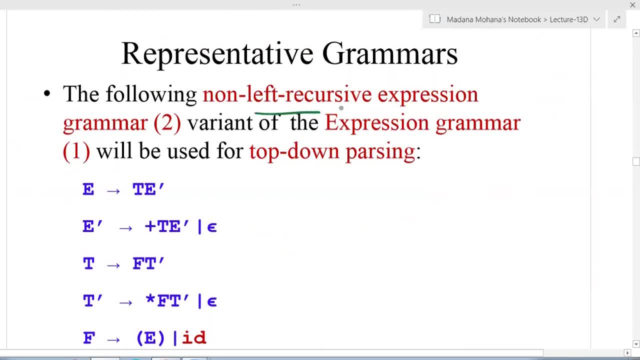 Then the grammar with left recursion Used for bottom up parsing. Now see one example of non left recursive grammar, The following: non left recursive expression grammar. Name it as two Variant of the above expression grammar. one Will be used for top down parsing. 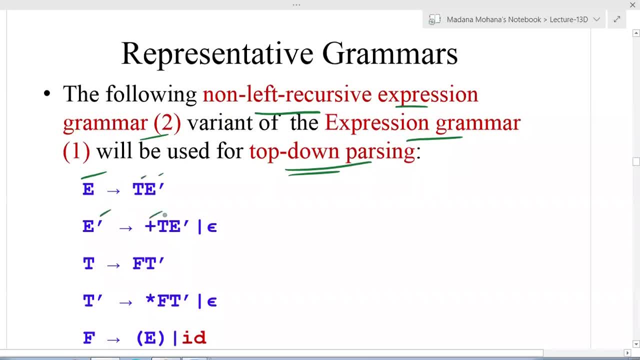 Now here you can see: TE derives TE dash Derives plus TE dash Arnold, Then TE derives FT dash, Then TE dash derives star FT dash Arnold. Then F derives E, within parenthesis RID. Now you can see this is not left recursive, because 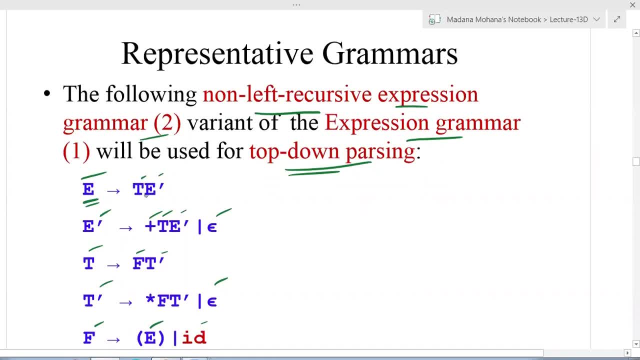 The left hand side variable Is not same as the right hand side of Left most variable. So here T not equal to T. Then here E dash, E dash not equal to plus. Then here TF, T not equal to F. 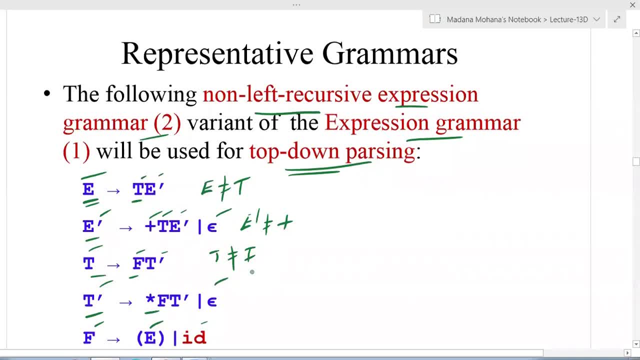 Then T dash, star, Only right hand side, left. Most simple, You can compare with the left hand side of the Variable of the each and every production. Here T dash not equal to star. Now here F, The first one is left parenthesis. 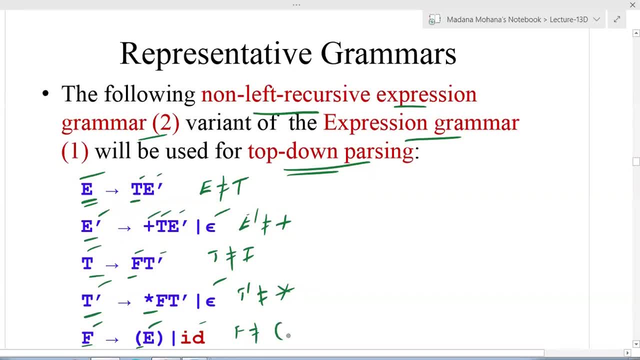 Don't see E, So therefore F Not equal to Left parenthesis. Therefore This is Non left recursive Here. left recursive is not this: This type of grammars are used for top down parsing. Then Another example. Let us see the following grammar three: 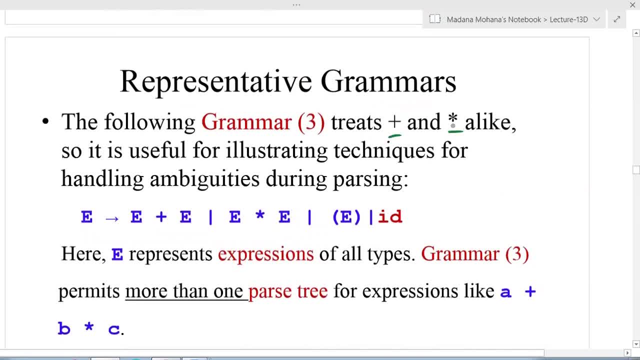 So treats plus and Asterisk alike. So it is useful for illustrating Techniques for handling ambiguities during parsing. So these type of Grammars are used For handling ambiguous grammars. So here you can see, Starting with the single. 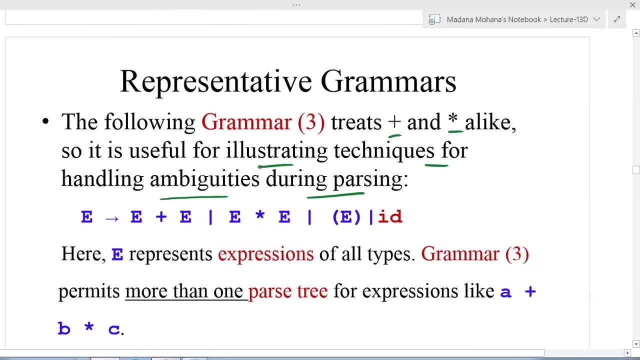 Variable. Here you have see The expression Plus E plus E, Then multiplication E into E, Then E within parenthesis or ID, So previously Grammar one Within parenthesis or ID. So here you can see The expression Plus E plus E. 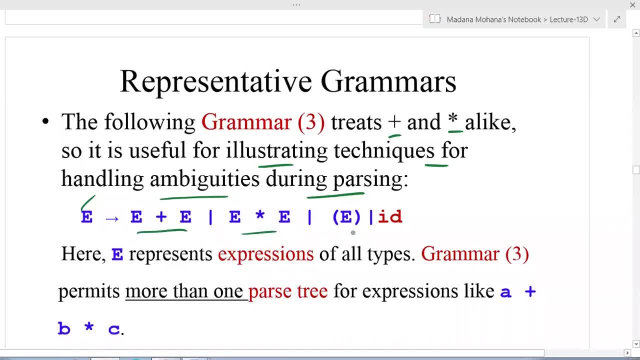 Then multiplication E into E, Then E Within parenthesis or ID, So previously Grammar one Within parenthesis or ID. So here you can see Grammar one With E to E. F Variables are there, But here only single. 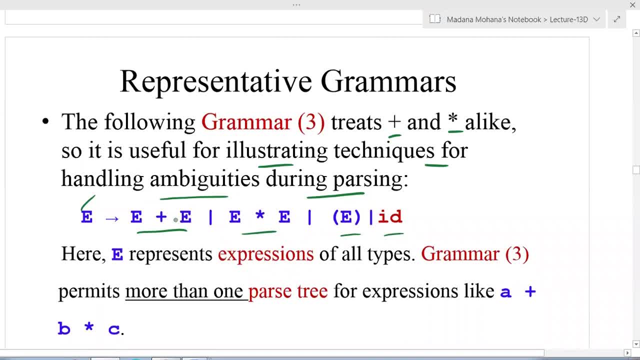 Variable With E. So these type of Grammars used For handling Ambiguous grammar. So here E represents Expressions Of all types. Then this grammar Three Permits more than one Parsity For expression. 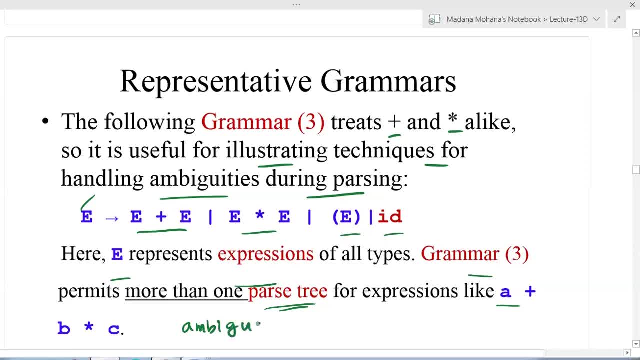 Like A plus B Into C, Then that is called as Ambiguous grammar- Ambiguous grammar. So in Automata theory We discussed The concept of Ambiguity, Then how to eliminate Ambiguity. Again, we will. 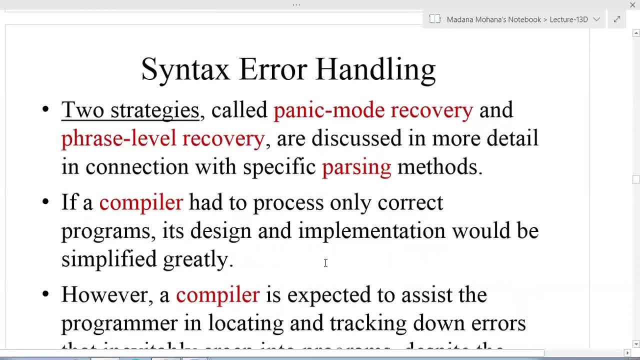 Recall those concepts Here. Then, Coming to Syntax error handling, So during Syntax analysis Or parser, It encounters Errors Which are called as Syntax errors, Here two strategies Called Panic mode recovery And Phrase level recovery. 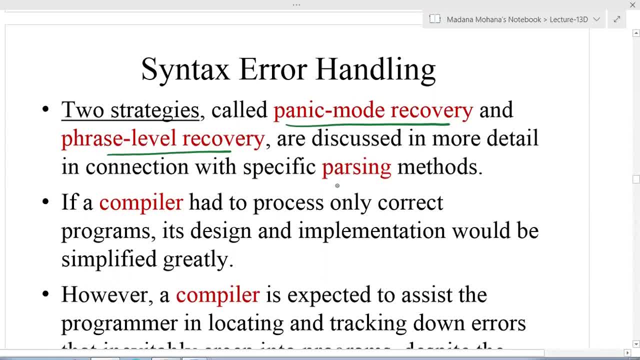 So, which are Discussed in more detail In connection with Specific parsing Method. If a compiler Had to process Only Five programs, Its design And implementation Would be Simplified Greatly. However, A compiler 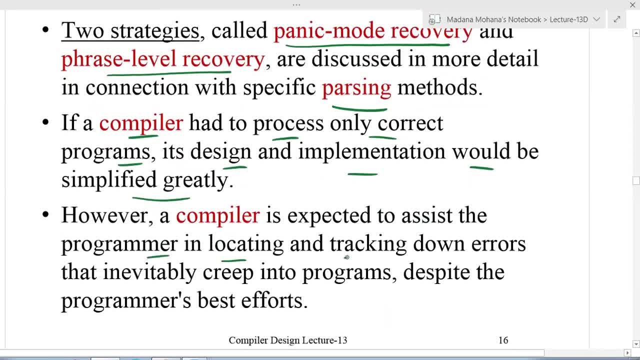 Is expected To assist The programmer In locating And tracking down Errors That Invitably Creep into Programs Despite The programmers Best Efforts. So Whenever Errors are Encountered, Then how to handle? 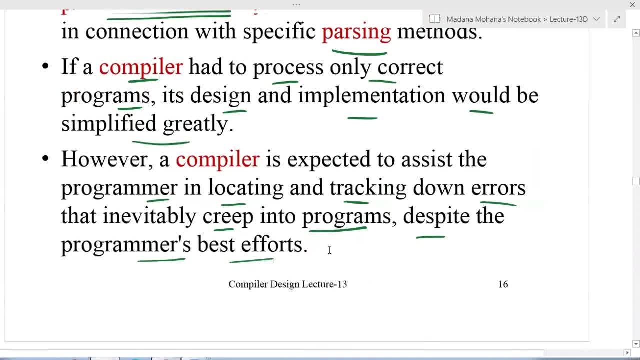 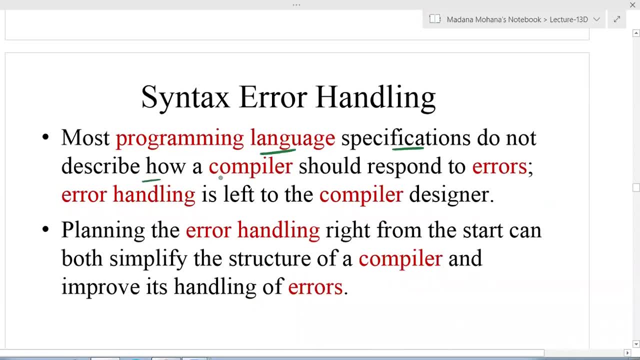 Those Errors: Panic mode recovery And Phrase level Recovery. Some other Techniques Also There. Most Programming Language Specifications Do not Describe How A compiler Should Respond To Errors, Whereas 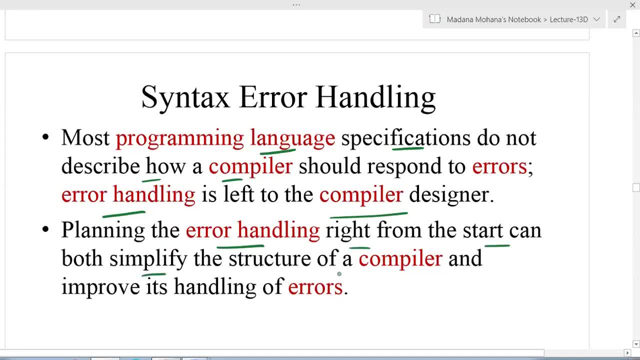 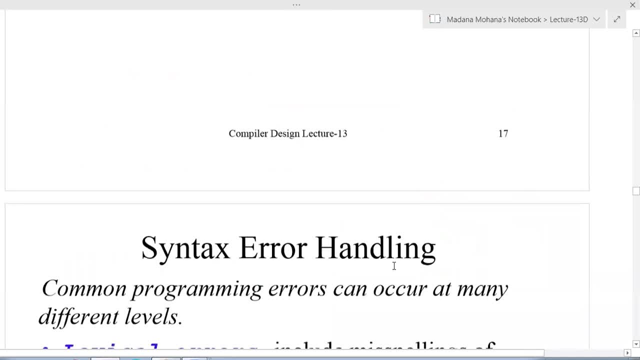 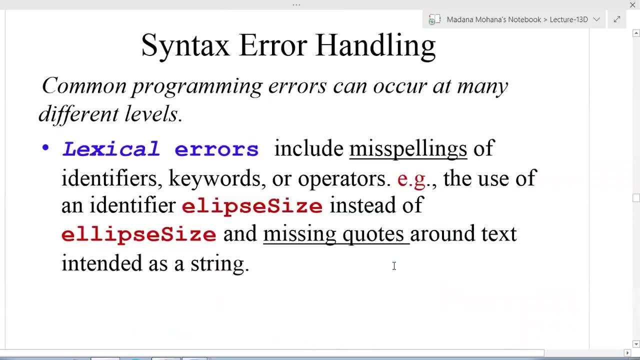 Error handling Is Left To The Compiler Designer To Errors. So That Is The Use Of Error Handling. Now Let Us See Various Types Of Errors. 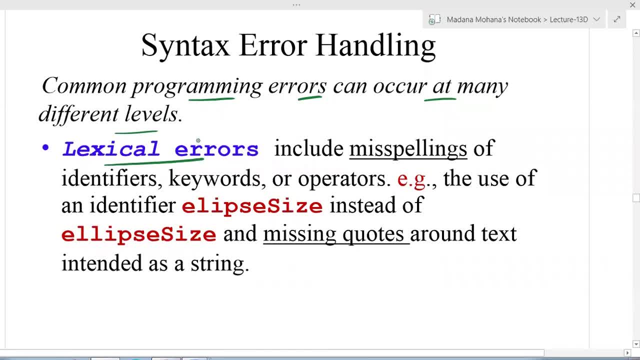 Common Programming Errors Can Occur At Many Different Levels. The First One Is An Identifier. Here You Can See E L, I, P, S E. 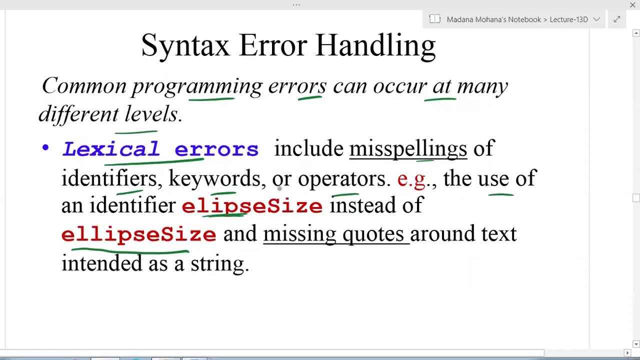 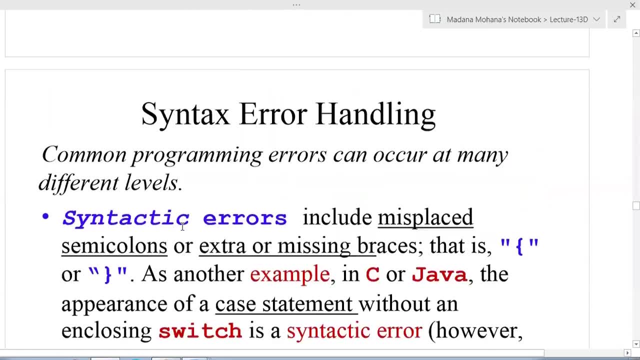 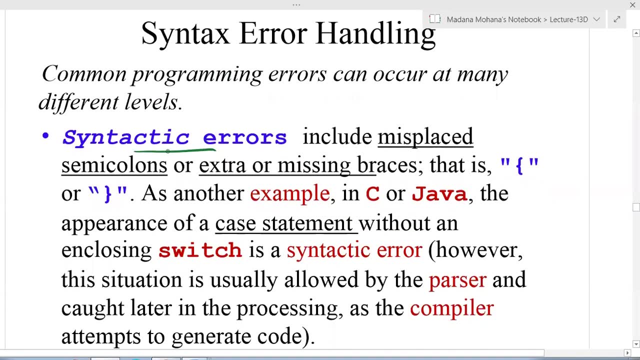 Size. So Instead Of Actually This Is Ellipse Size Here. This Is Misspelled And Missing Quotes Around Text Analysis Or Parts: Syntactic Errors. 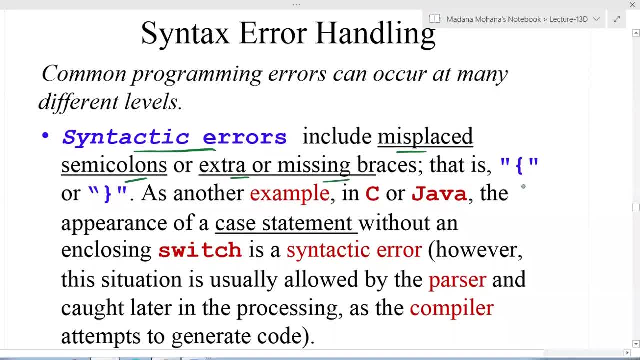 Also Include Misplaced Semicolons Or Extra Or Missing Braces. So That Is The Brace, Like This Open Brace Or Closed Brace It May. 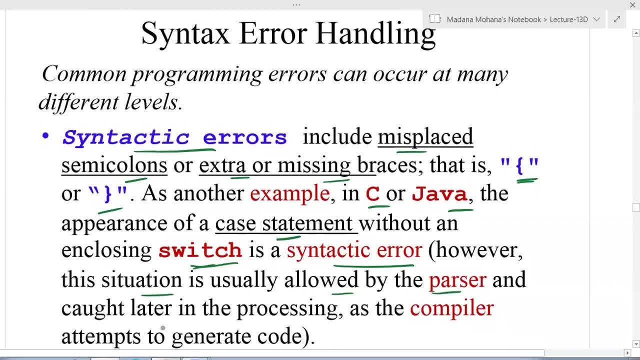 Be A Part Of The Processing As The Compiler Attempts To Generate Code. So Here A Switch Case Encloses: Are Not There? So Within The 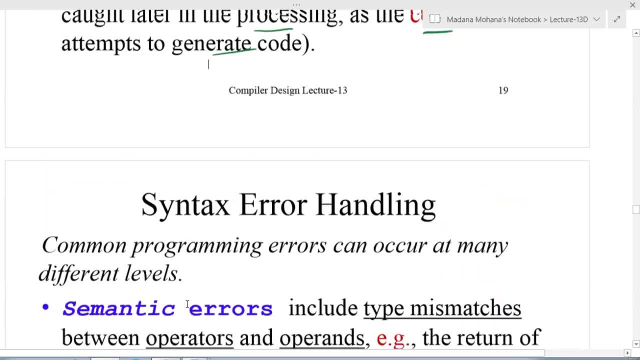 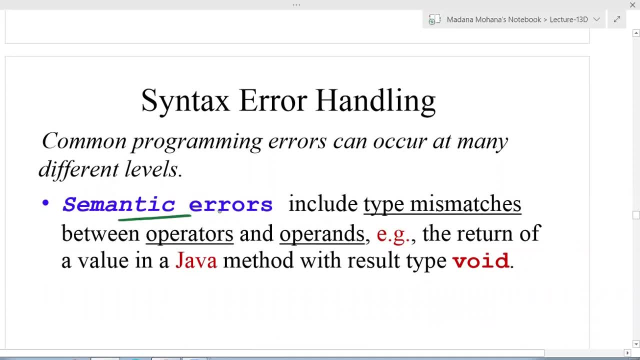 Function With Arguments. So Then The Type Of Common Errors Is Called A Semantic Error, Which Is Related To The Third Phase, Semantic Analysis, Which Includes 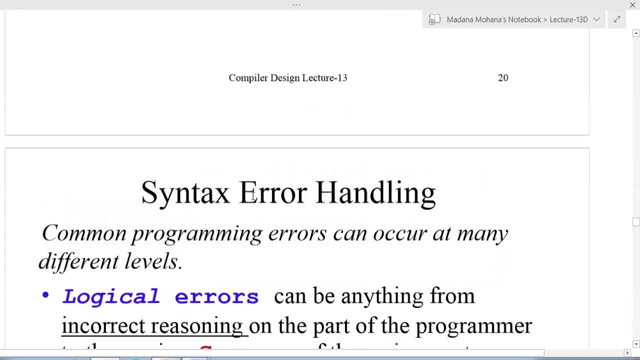 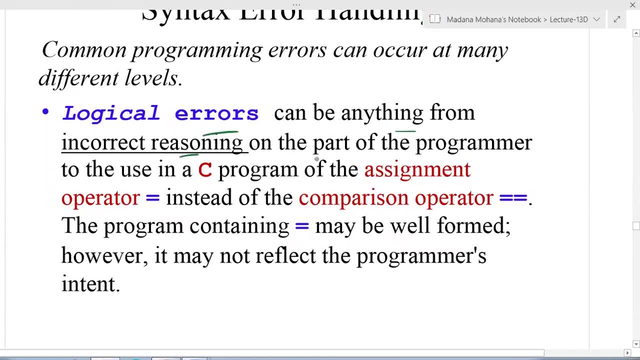 Type Mismatches Between Operators And Operants For Logical Errors Can Be Anything From Incorrect Reasoning On The Part Of The Programmer To Use In 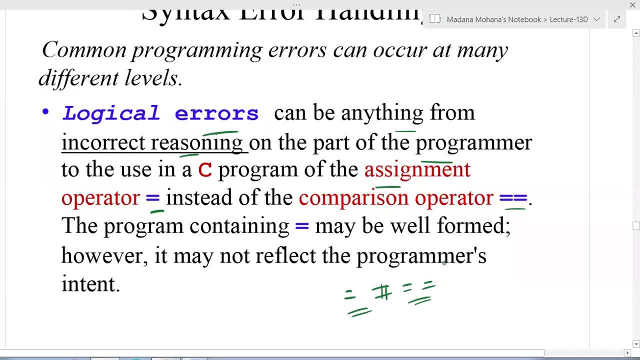 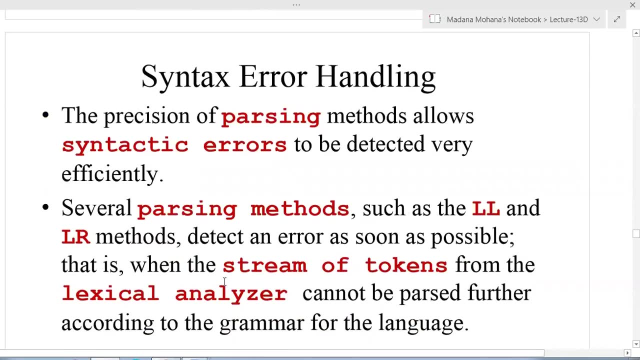 A, C Program Of The Assignment Operator Equal, Instead Of The Comparison Of Logical Errors, Then These Are All Commonly Used Programming Errors With Various 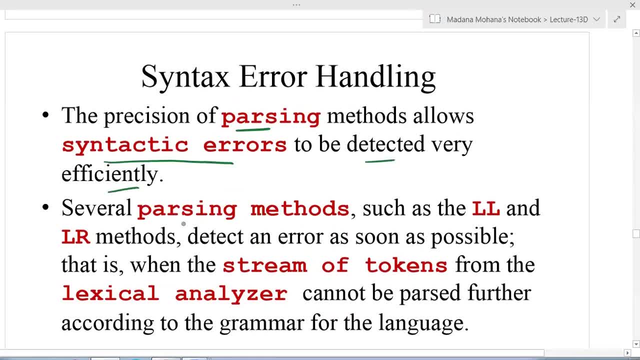 Phages, Then The Precision Of Parsing Methods Allows Syntactic Errors To Be Detected Very Efficiently. Several Errors Can Not Be Parsed Further According. 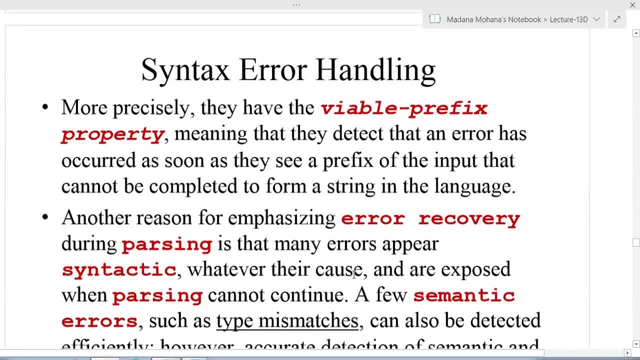 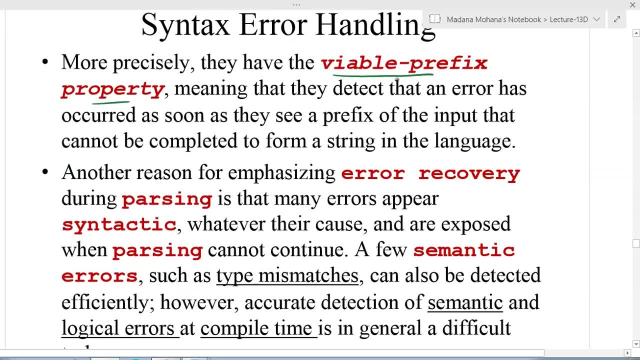 To The Grammar Or The Language At The Time. These Errors Are Syntactic Errors Are Occurred Then. More Precisely, By Considering Variable That: 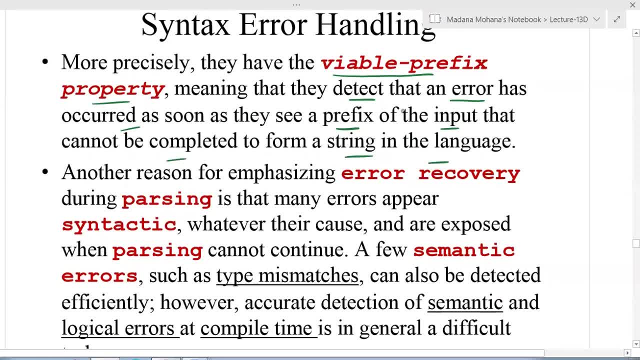 Can't Be Completed To Form A String In The Language Immediately By Seeing The Prefix Of The Input String. So Another Reason For Emphasizing. 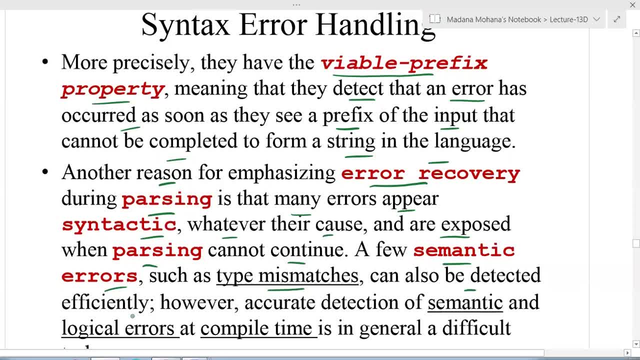 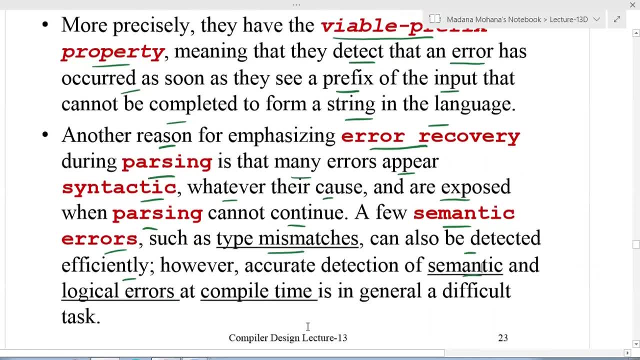 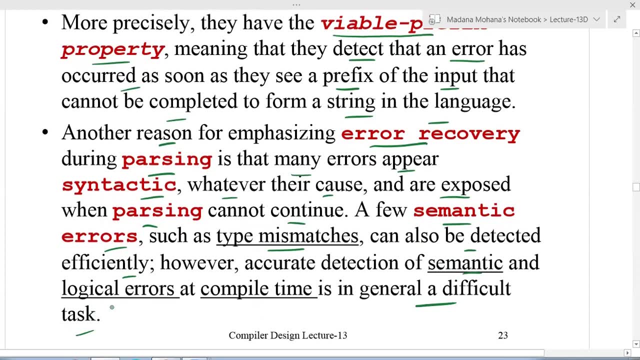 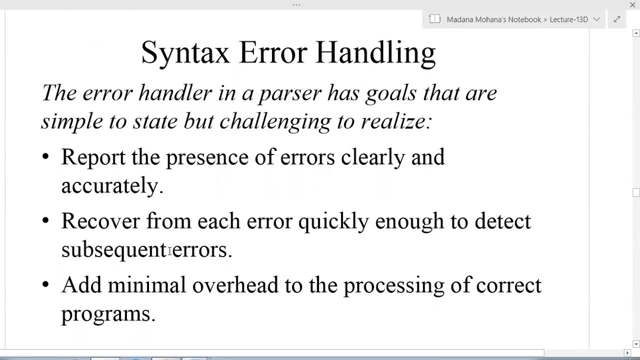 Error Recovery During Parsing. However, Accurate Detection Of Semantic And Logical Errors At Compile Time Is In General A Difficult Task To Handle. Semantic And 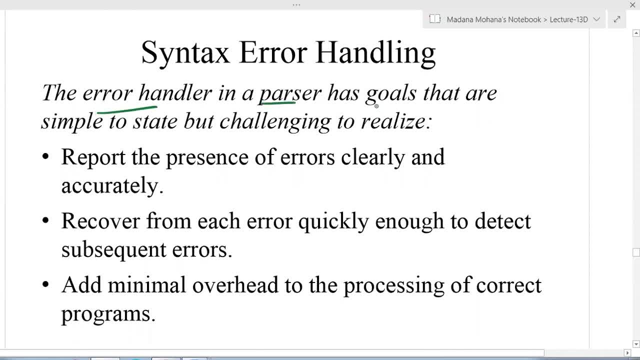 Logical Errors During Compilation. That Is Very Difficult To Realize. So What Are The Error Handler? Goals In Parsing Or Syntax Analysis. That Means The 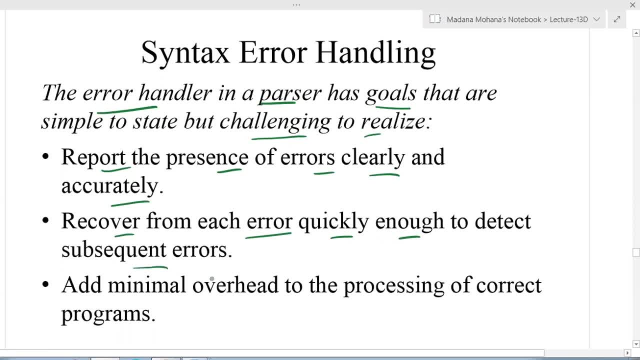 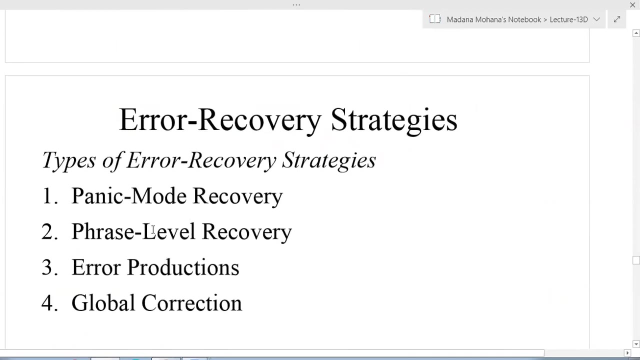 Task Needs To Be Performed- Report The Presence Of Errors Clearly And The Task To Handle By The Parser In Error Handler During Syntax Errors. 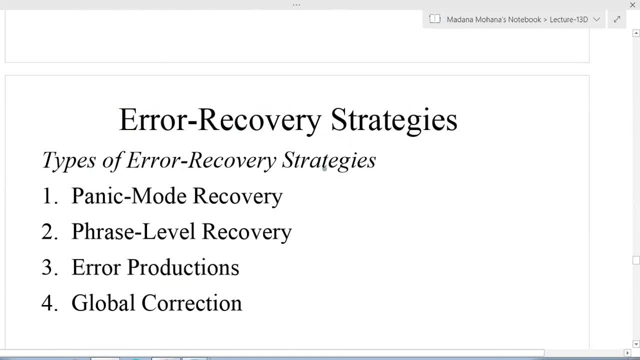 Then Let Us See The Error Recovery Strategies, With The Detail Explanation, The Types Of Error Recovery Strategies, In Addition To These Two Error Recovery Strategies. 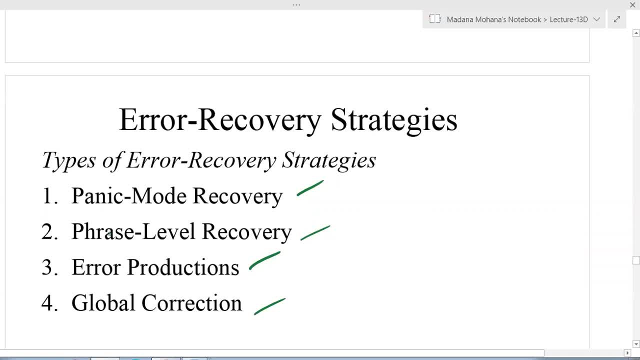 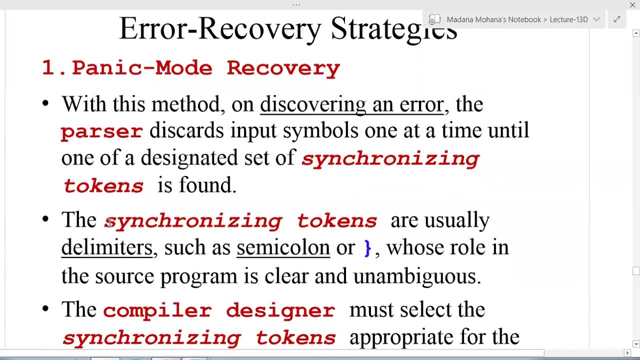 Also Included Here. Those Are All Error Productions And Global Correction. Finally, These Four Error Recovery Strategies Are Used To Error With This Method On Discovering. 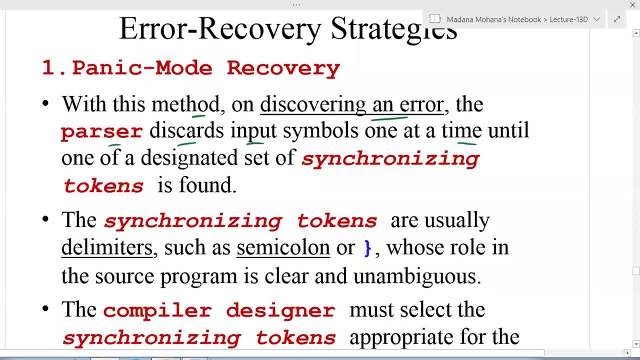 An Error, The Parser Discards Means, Removes Input Symbols One At A Time, Until One Of A Designated Set Of Synchronizing Token Is Unambiguous. 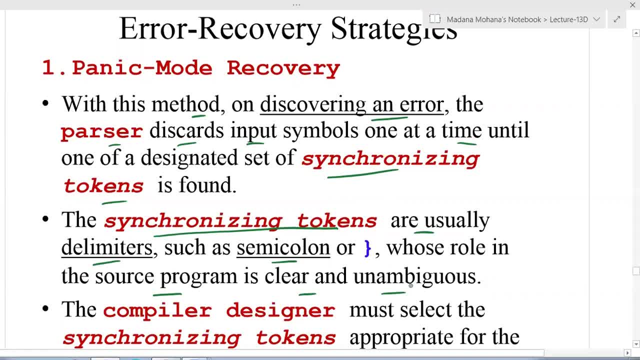 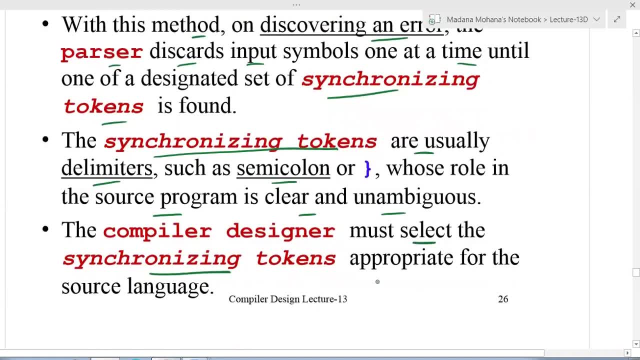 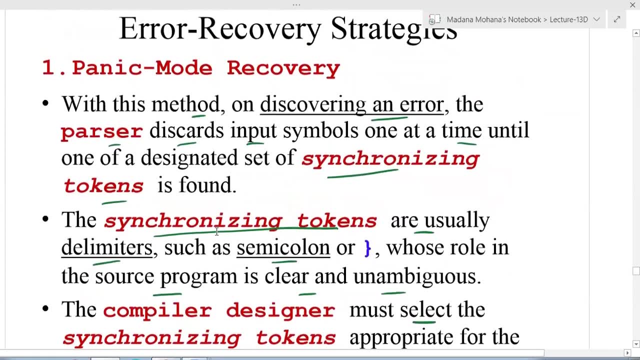 Means With, Without Ambiguity It Clear? Then The Compiler Designer Must Select The Synchronizing Tokens Appropriate For The Source Language. So These Are: 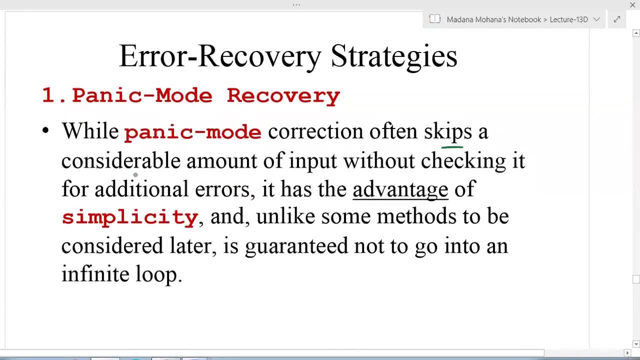 All The Various Steps In Input Without Checking It For Additional Errors. It Has The Advantage Of Simplicity And, Unlike Some Methods To Be Considered. 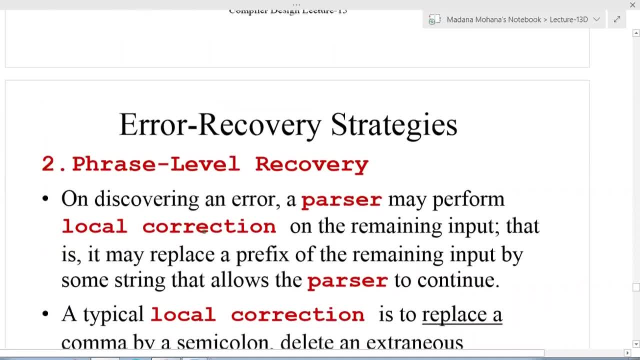 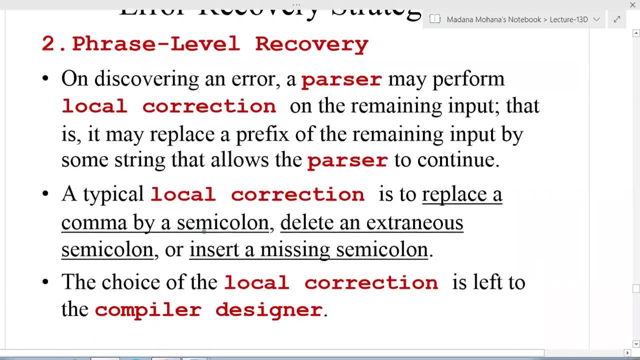 Later Is Guaranteed Not To Go Into An Infinite Phase Level Recovery. On Discovering An Error, A Parser May Perform Local Correction Within That Particular. 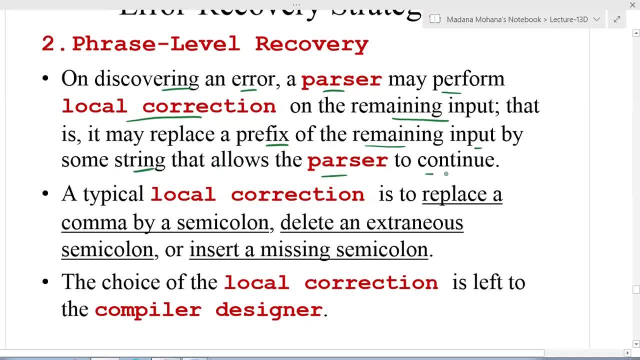 Method Within That Particular Program. So On The Remaining Input That That Is Replaced With By A Semicolon, Then Delete An Extranet Semicolon. 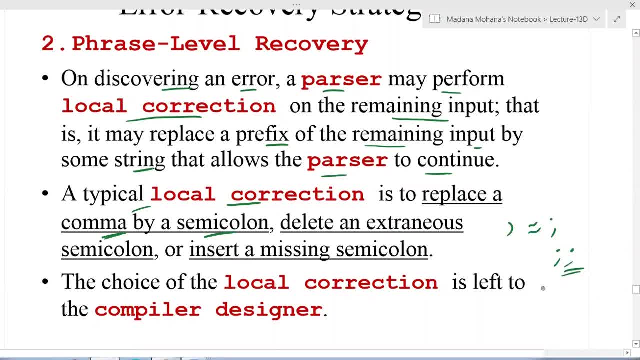 Suppose We Have Two Semicolons, So Remove The Extranet Semicolon, Then Inserting A Missing Semicolon, Suppose Here, Print F Local Correction. 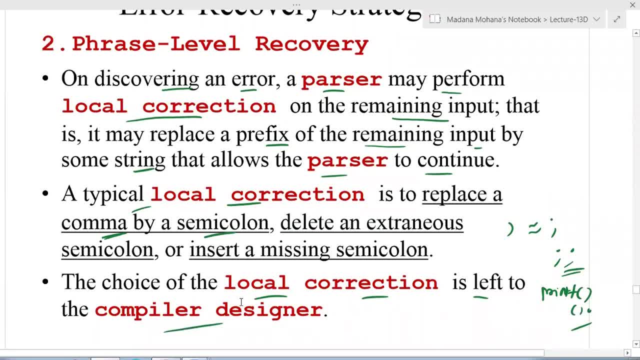 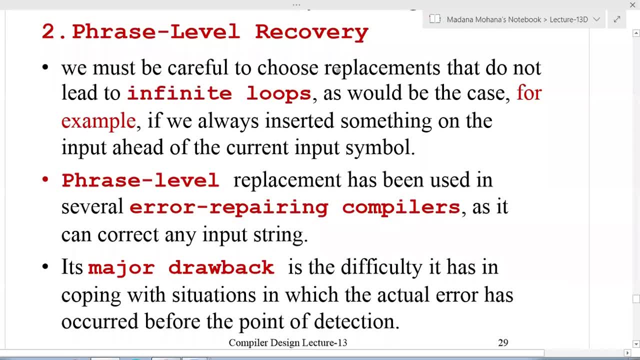 Is Left To The Compiler Designer Later, So Based On The Requirements. So Then Here We Must Be Careful To Choose Replacement That Do Not. 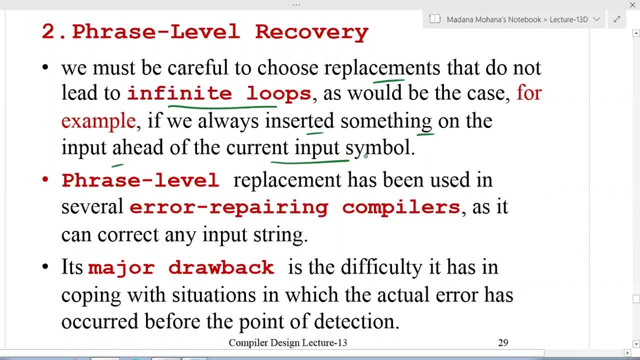 Lead To Take Care Of Whether It Leads To Any Infinite Loop Or Not, Then Phrase Level Replacement Has Been Used In Several Error Repairing. 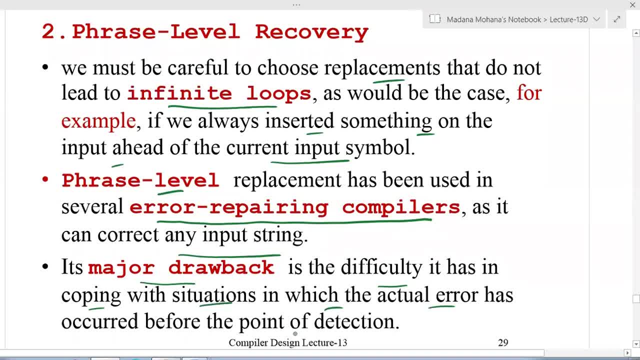 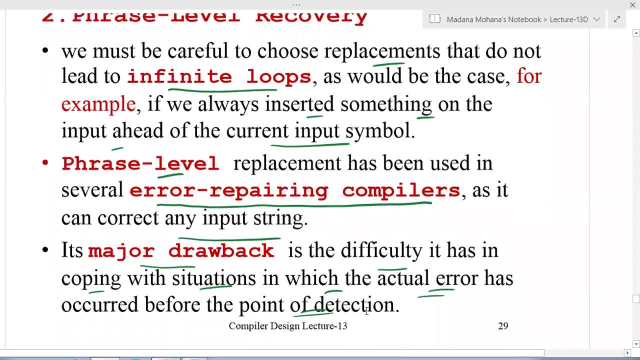 Compilers, As It Can Correct Any Input Coping With Situations Arranges In Which The Actual Errors Has Occurred Before The Point Of Detection. 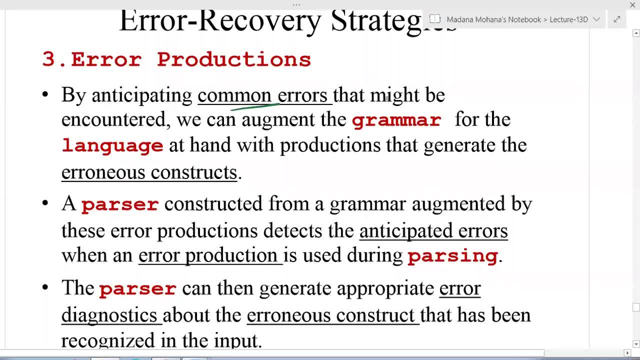 This Is One Of The Major Drawback Of Phrase Level Recovery, Then Coming To The Errorness Construct, So Here We Will Substitute Error Productions To 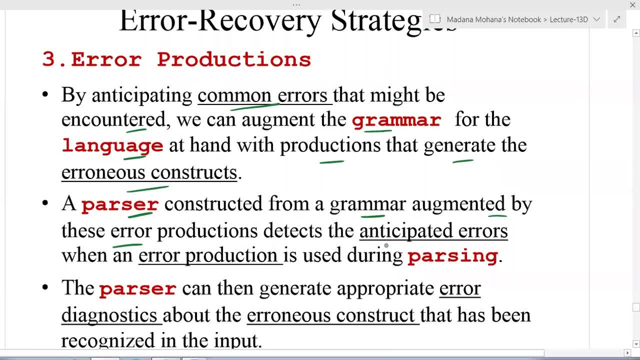 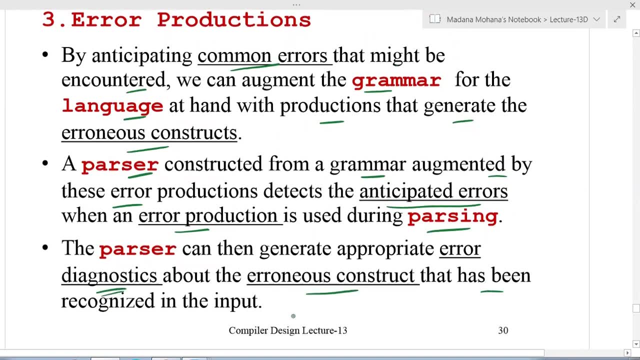 Hand To Recur, To Recur Or Rectify The Errors. A Parser Constructed From A Grammar Augmented By That Has Been Recognized In The. 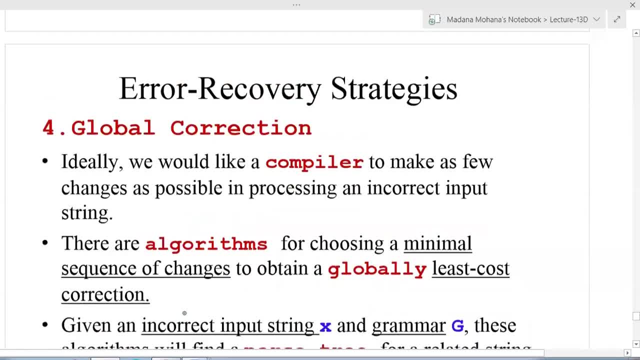 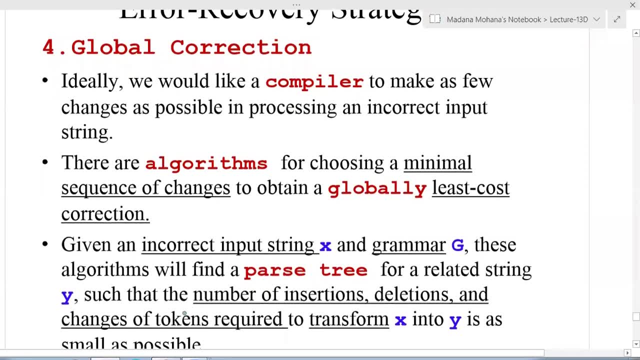 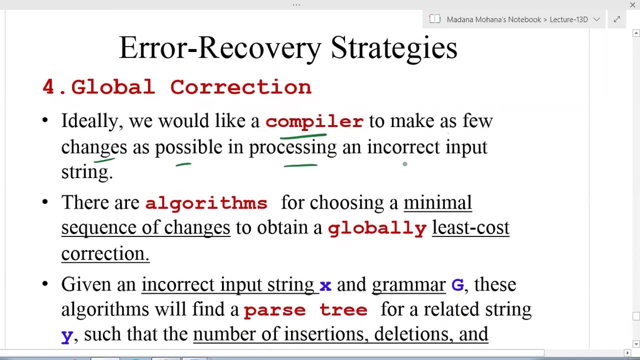 Input, So By Diagon, Diagon Sizing, By Including Error Production, That Is Error Production Status, Then The Last Mechanism, Global Correction. So Ideally Here, 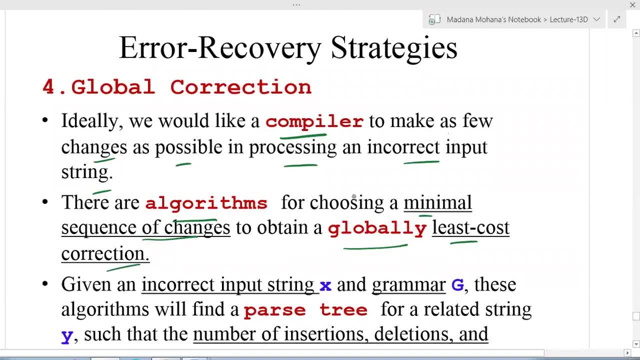 Obtained Globally With Least Cost Correction, Global Correction So Commonly To That Entire Program. So You An Incorrect Input, String X And A, Grammar. 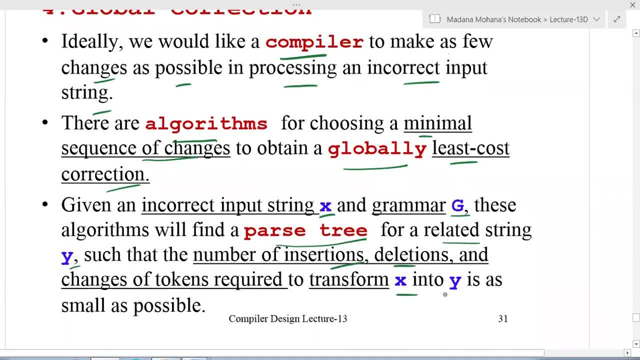 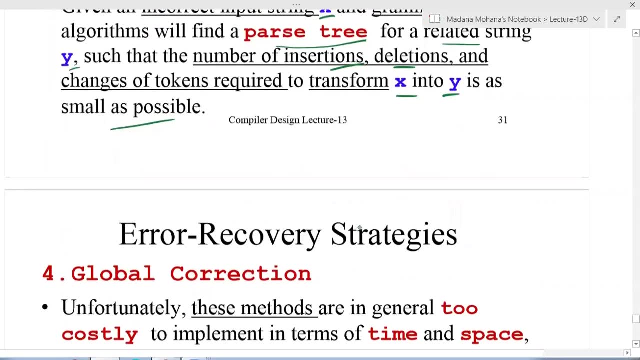 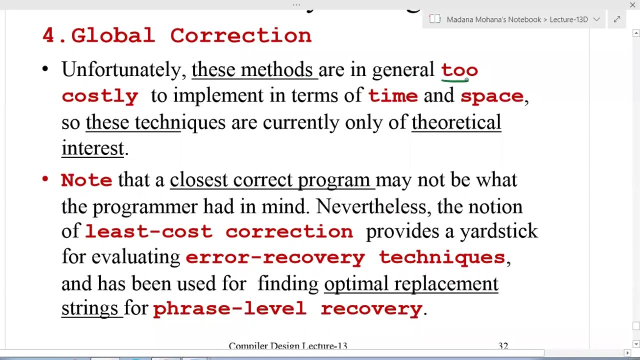 G These Algorithms Will Find Is As Small As Possible. So This Is The Transformation For Correcting Globally. So This Is Global Correction Strategy Now. 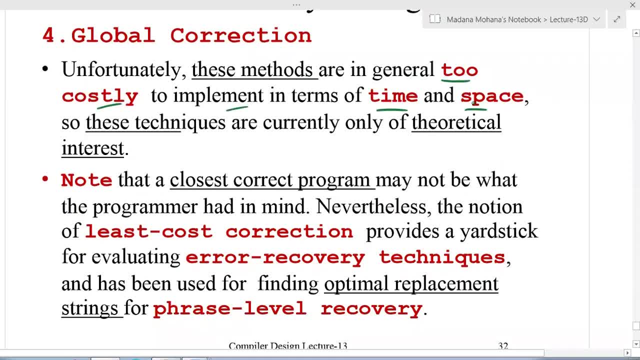 Here Let Us See Some Of The Drawbacks Of Strictly So We Can't Use More, So Here Let Us See One Of The Observation. 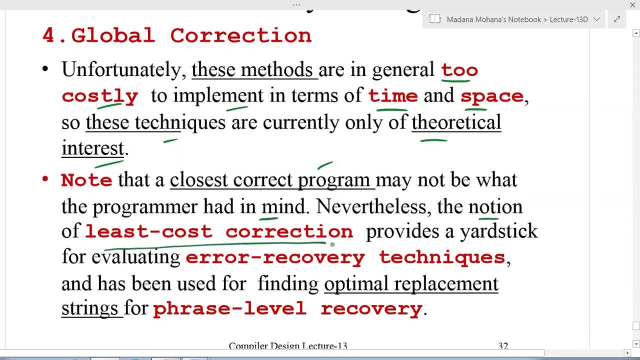 A Closest Correct Program May Not Be What The Programmer Had In Mind. Nevertheless, Replacements, Things For Raise Level Recovery. So, Even If We Can, 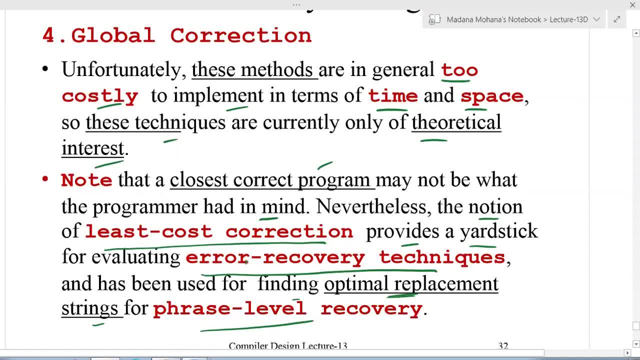 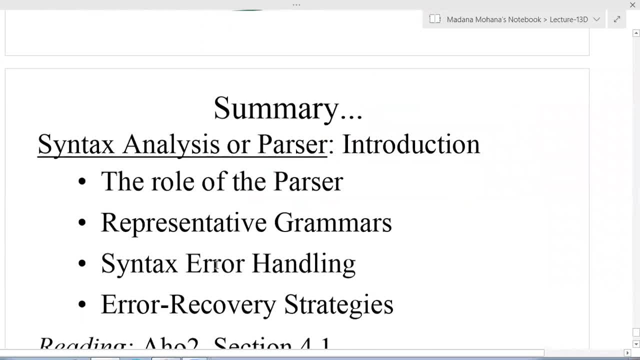 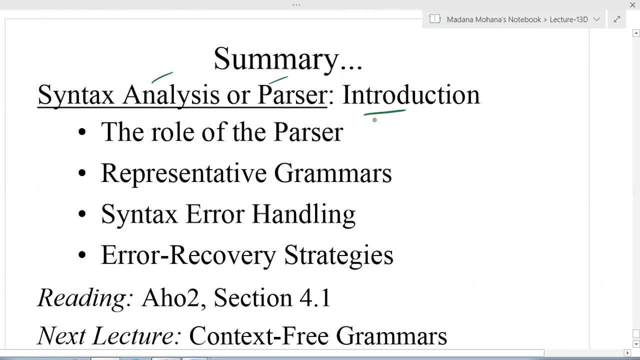 Use Any Of These, Only Optimal Replacements Of Strings Only. So These Are Some Of The Cousins We Have To Introduction To Syntax Analysis Or 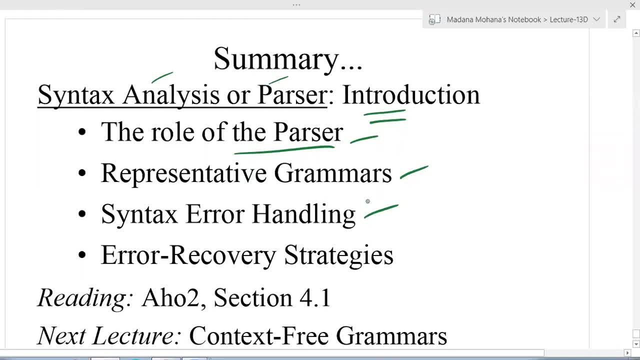 Purser, Then The Role Of The Purser, Then Representative Grammar, Then Syntax Error Handling. Here We Discussed Various Types Of Errors, Then Various Types. 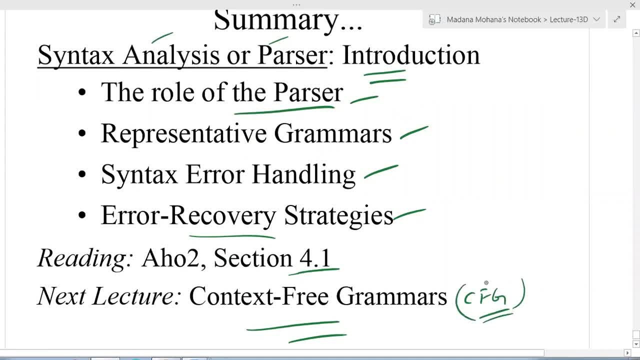 Of Errors Of Errors, The Form, Language And Automata Theory. So Again, We'll Recall All: The Concept, Definition Of The Grammar, Derivation, Then Ambiguity. Then Elimination Of Ambiguity.